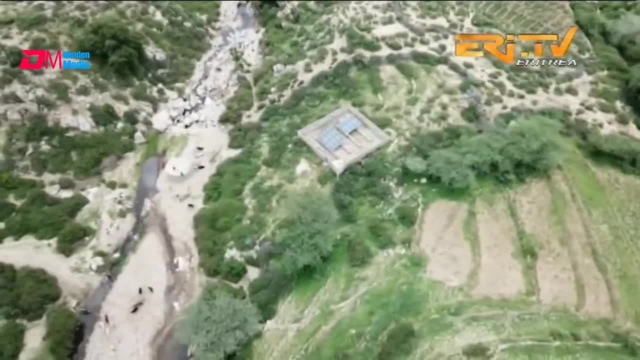 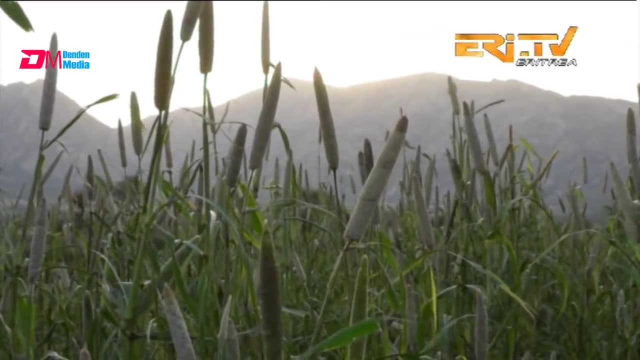 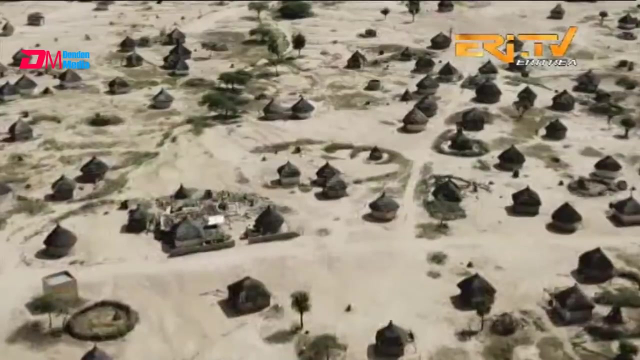 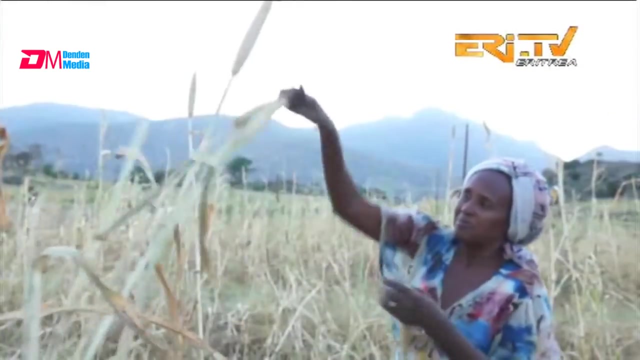 The US$6 million project, implemented by the Ministry of Land, Water and Environment and the Ministry of Agriculture, has been operational since 2013 in two sub-zones, namely Habero and Hamilmalo of the Ansuwa Region, with average annual rainfall being 190 mm and 367 mm for Habero and Hamilmalo. 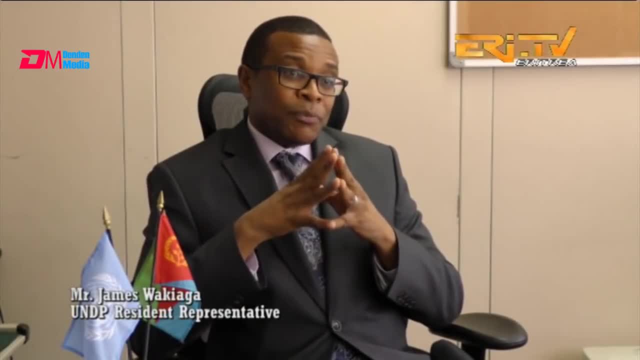 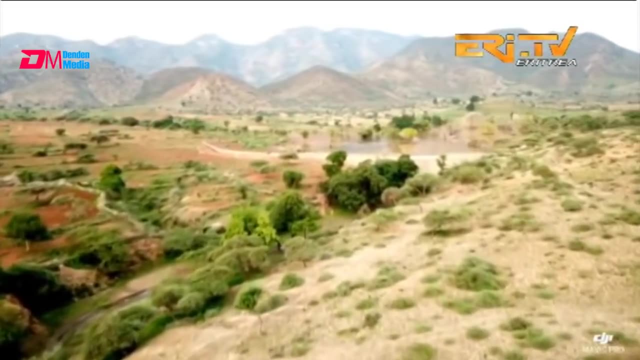 respectively. It is basically an adaptation program to try to address the issues of the climate change action in Eritrea. As you know, all countries are facing this challenge of climate change And it's impacting on lives. it's also impacting on the economy. 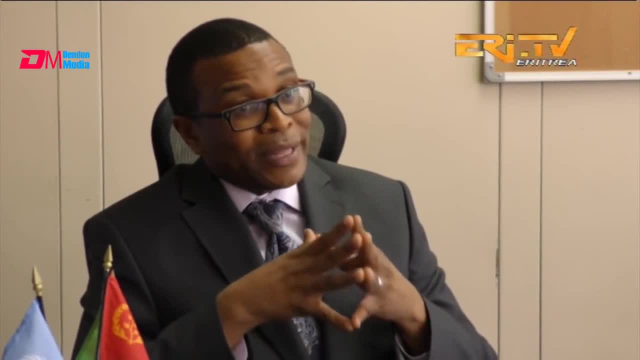 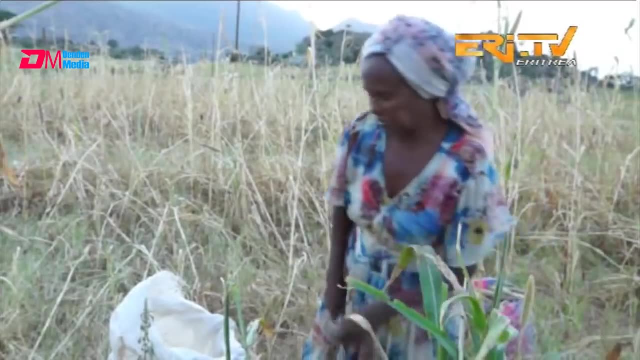 and it's part of the SDG, Sustainable Development, Goal 13,, which is on climate action. The objective of the program is to increase community resilience and adaptive capacity to climate change through an integrated water management and water management system. and adaptive capacity to climate change through an integrated water management and water management system. 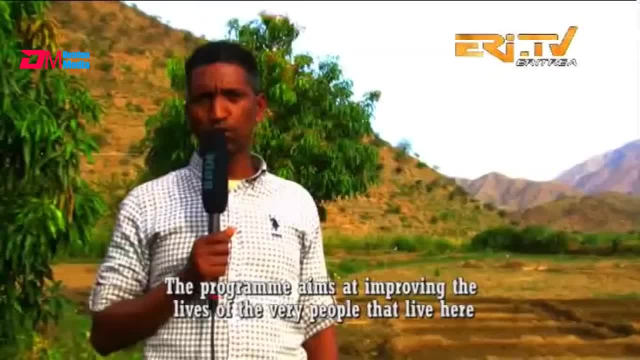 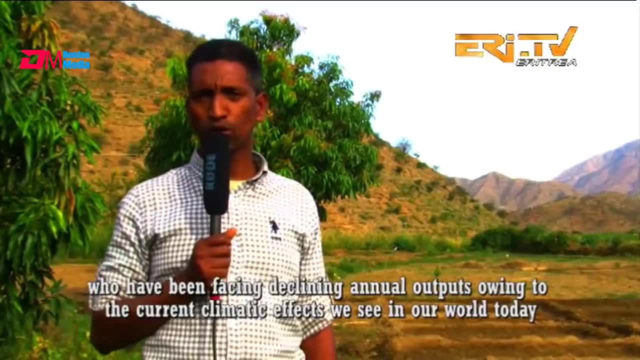 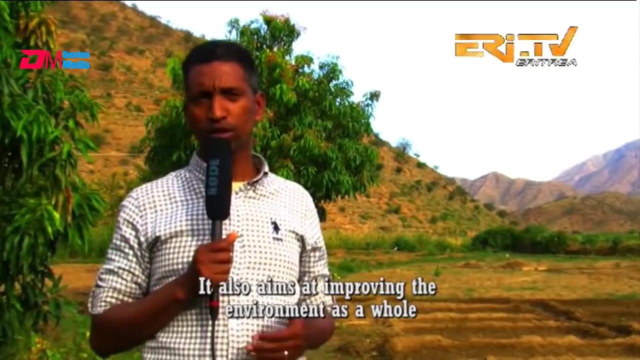 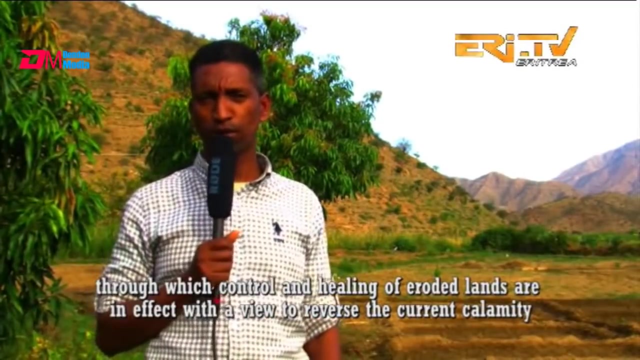 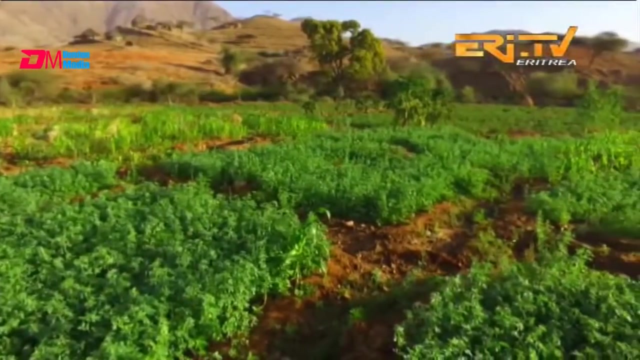 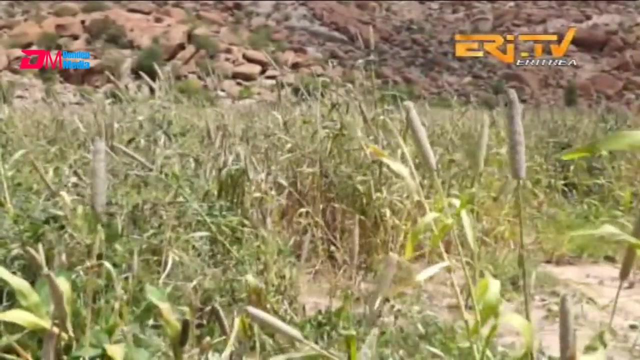 and agricultural development approach. With the development approach, it could hand over some of the desires. It could hand over some of the desires. It could hand over some of the desires, and land, water and environment worked closely and effectively to provide quality support and input to ensure timely implementation and 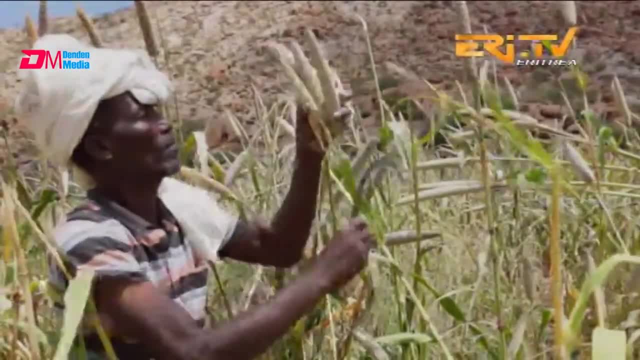 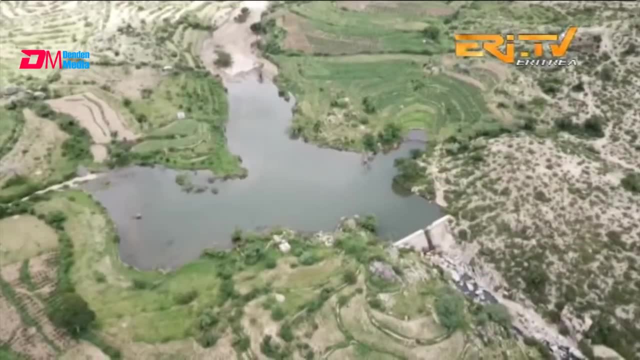 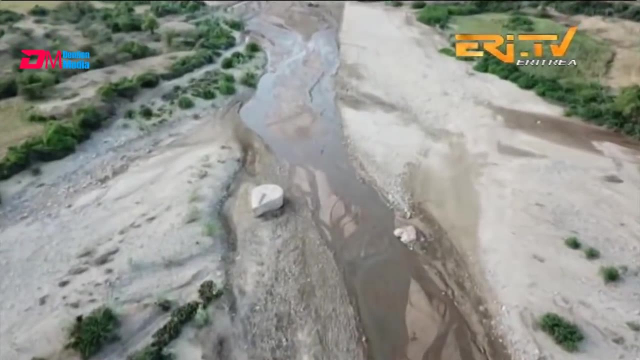 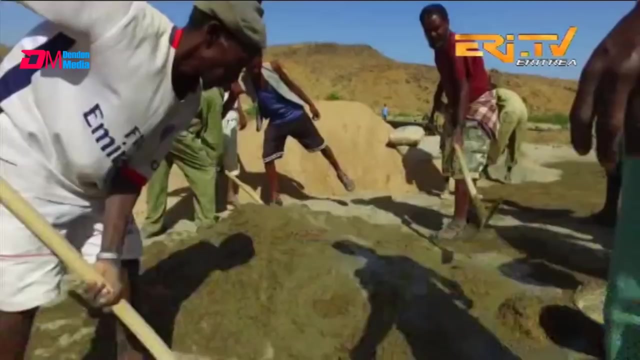 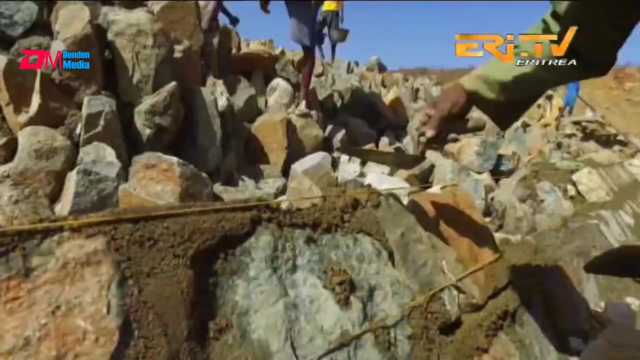 accomplishments of the program's outputs and outcomes. the construction of divergent structures and associated irrigation technologies, such as construction of dams, micro dams and check dams, have complemented the increase of water availability and erosion control. through groundwater recharge, rainwater harvesting, irrigation and soil in water conservation activities, the program was able to increase the availability of. 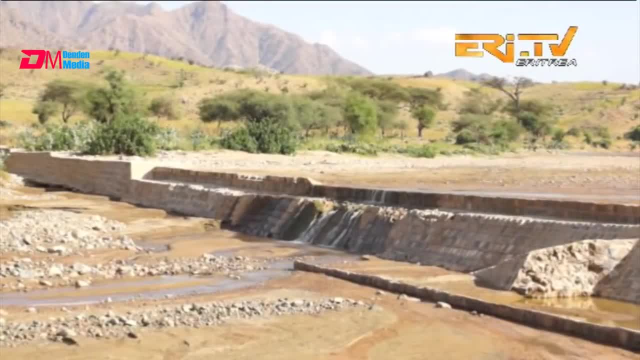 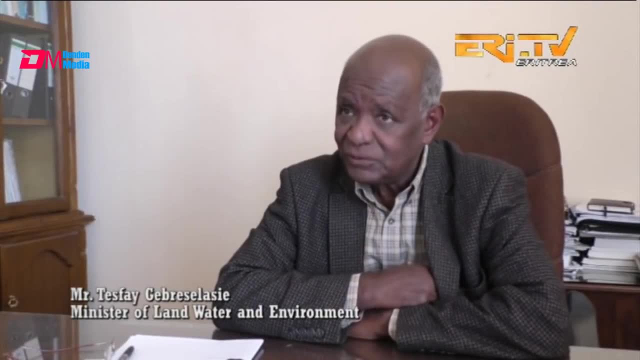 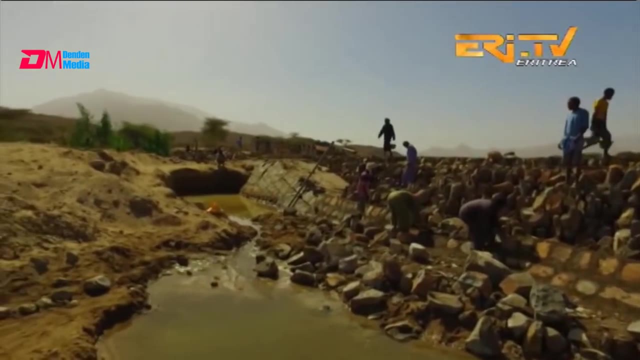 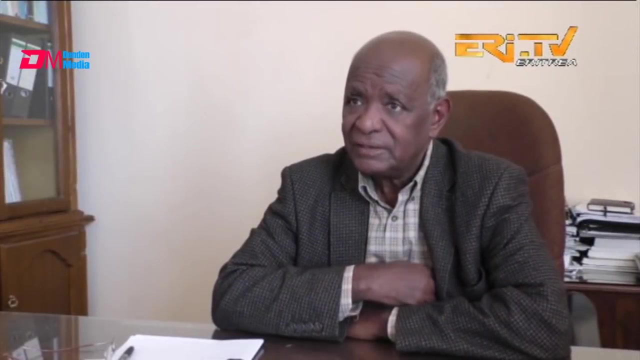 water by about 1 to 2 million cubic meters of water. this projects have been well improvement of the food supply of the community in terms of quantity and quality, and this was possible thanks to the construction of micro dams, seasonal river flow diversion structures, which need to. 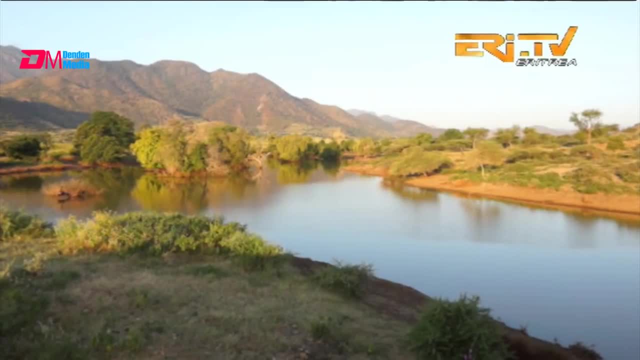 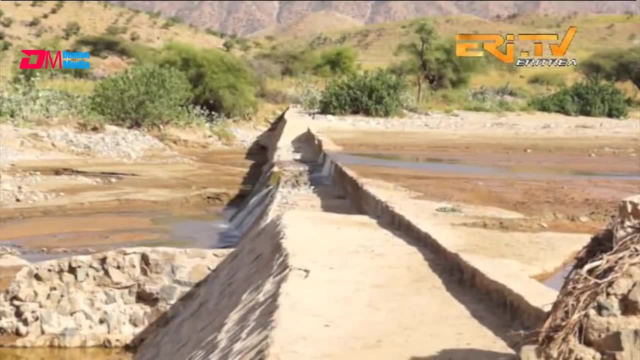 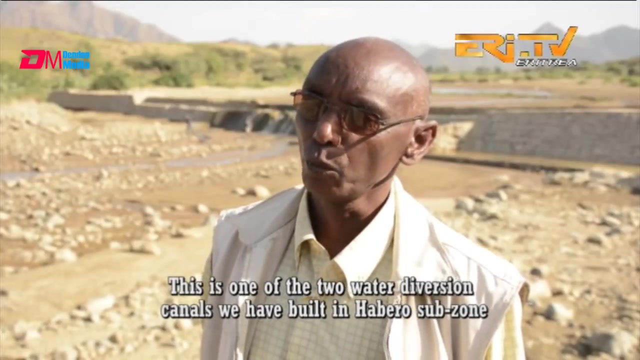 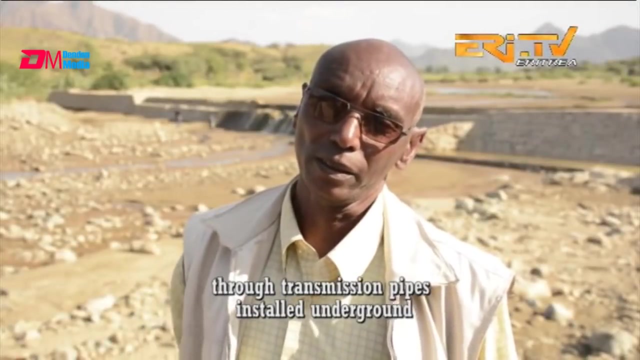 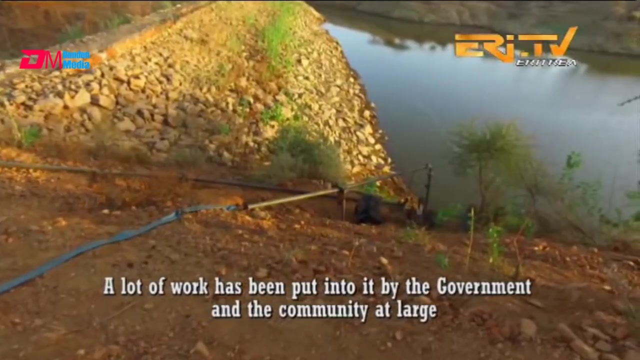 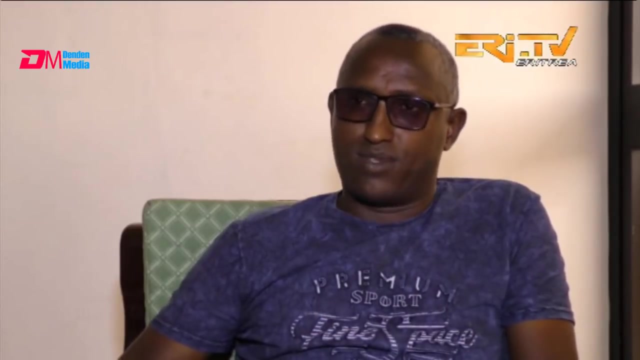 develop irrigated agriculture. the project has been working with vulnerable groups, including small-scale farmers, agro pastoralists, pastoralists and rural women. in relation to climate change-induced problems, yeah, solar electric. This is the most drought-stricken area and the people, the life mode of the people was: 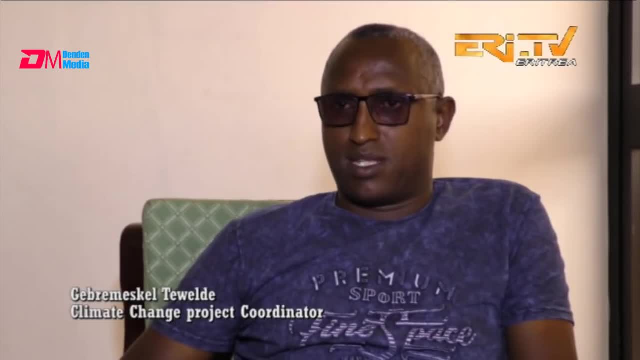 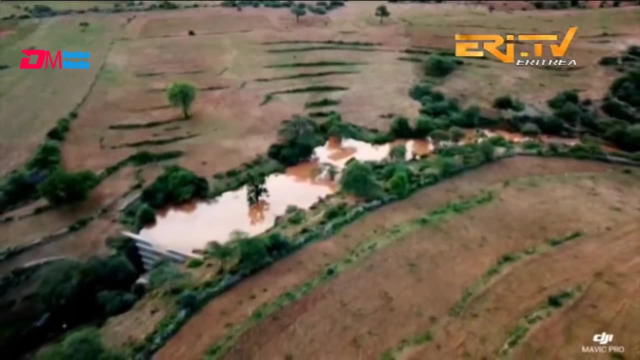 pastoralists. so through this project I think they become sedentary farming, meaning that they are trying to produce twice in a year or three times in a year. So we are trying to mitigate this climate problem, so we are pushing the farmers to 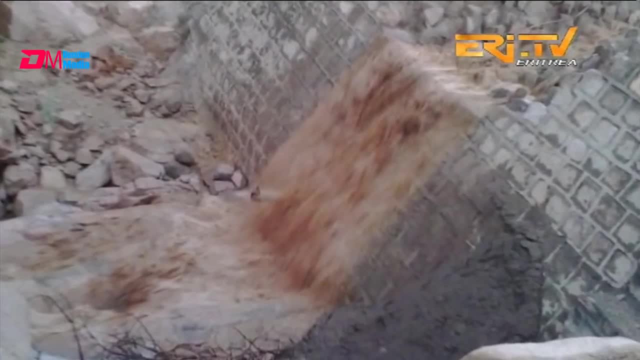 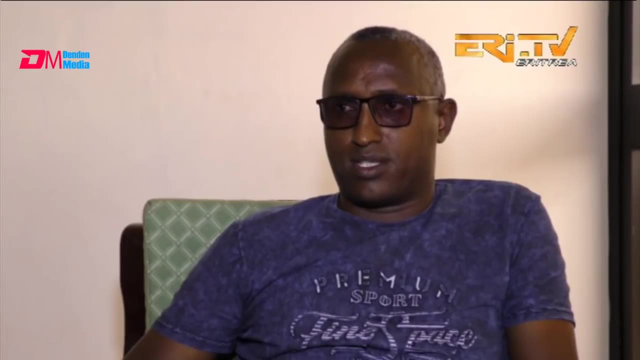 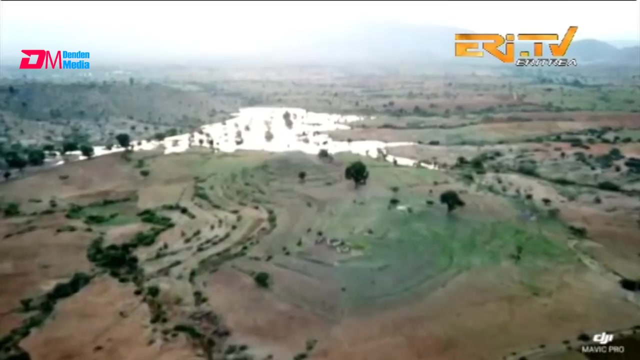 use this solar-driven engine. So by now, almost around 13 hectares has been irrigated with solar system. the rest they are. using this flood diversion structure And again using this outcome one, we are building different dams and check dams. We are able to harvest almost more than 2 million cubic meters of water. 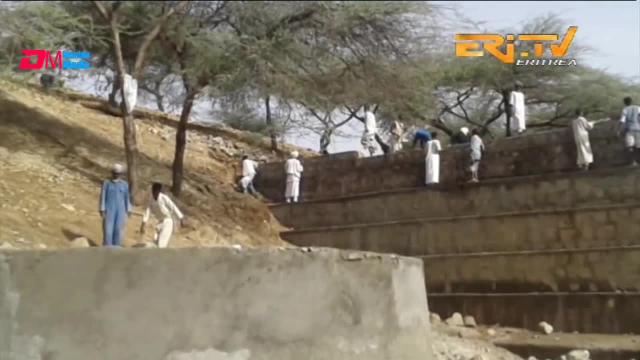 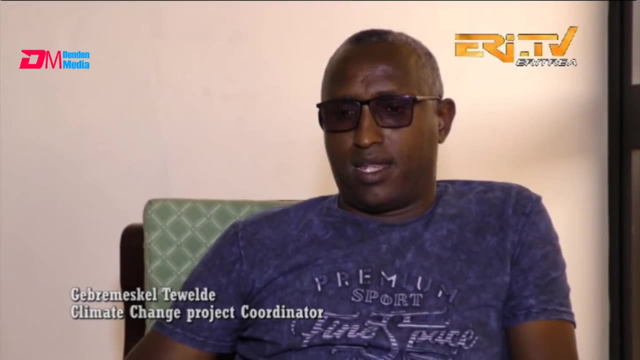 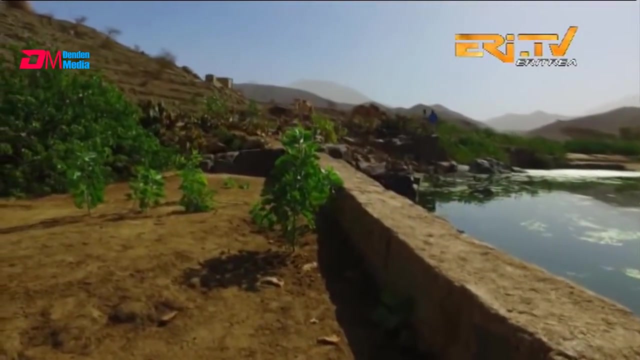 So within these two cubic meters I think the farmers they got a good chance to get water easily, just using the shallow water, And also not only for irrigation purpose but domestic water supply. All in all, in the outcome we have done a very satisfactory activity at works. 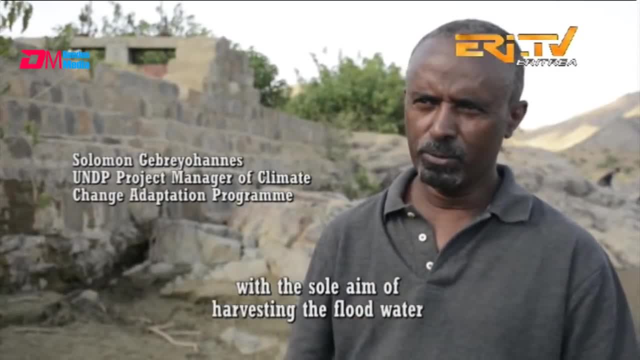 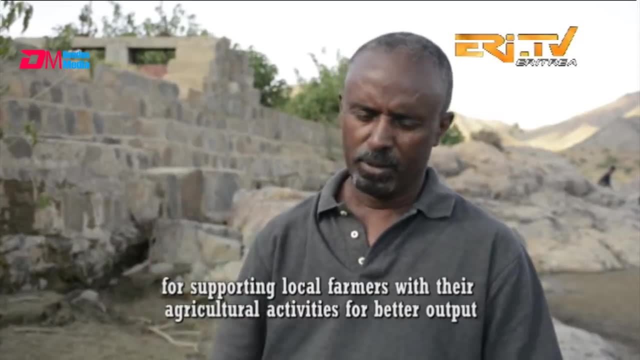 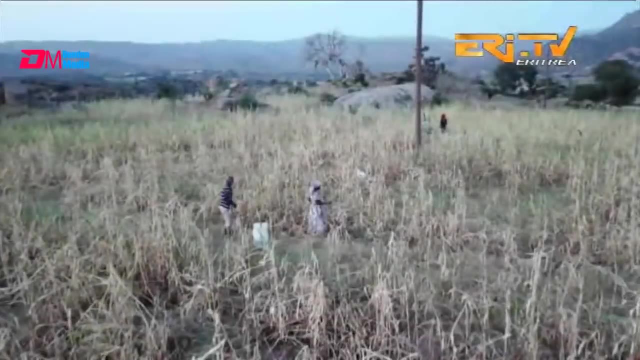 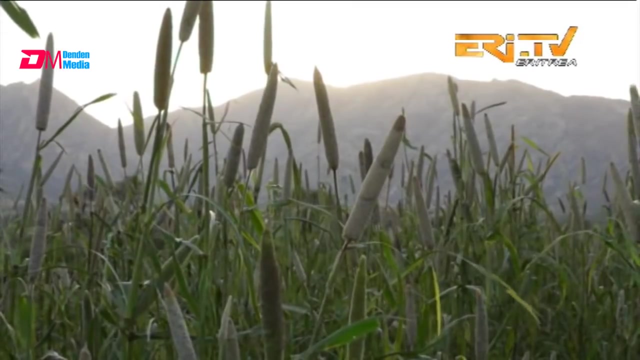 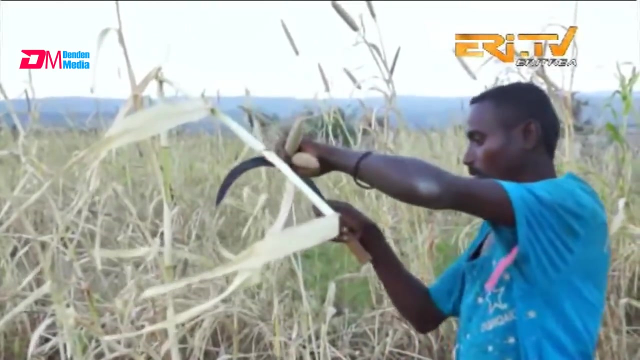 The climate resilient agricultural technology, such as the distribution of improved and drought resilient pearl millet seeds, have been introduced through this program in order to help farm households secure food and nutrition, income and employment, as well as provide marketable surplus for urban dwellers. 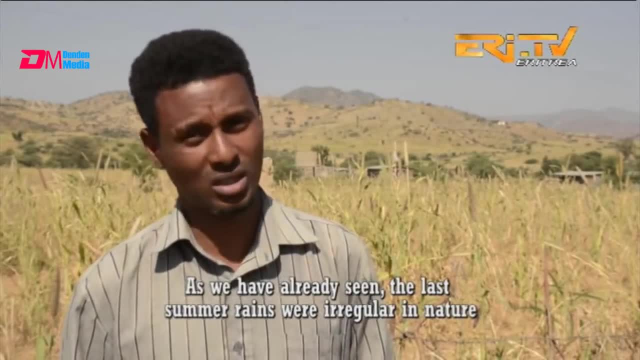 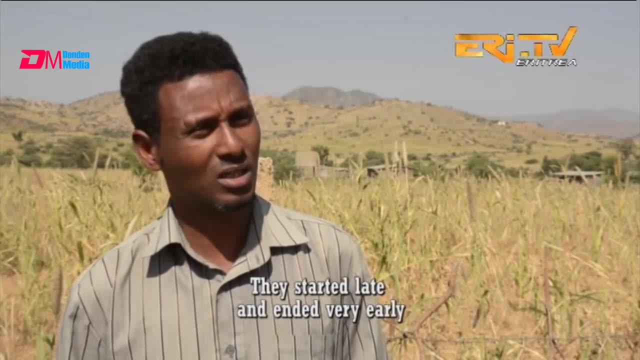 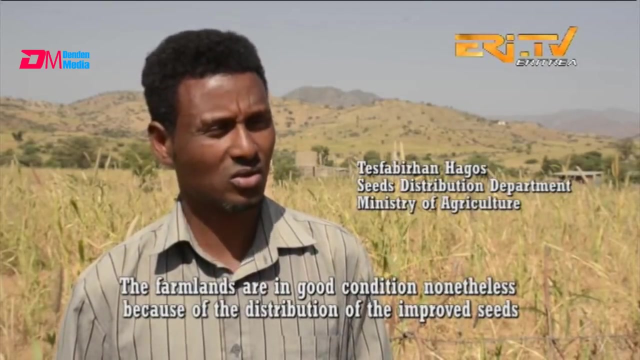 The program has been implemented in several regions in the region, including the Kufu Kufu region and the Jammu region. We areGAI and other organizations have been working with the program to help our farmers secure food and nutrition and to get the best results. 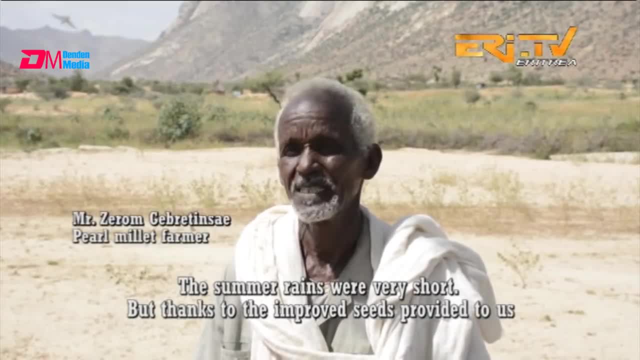 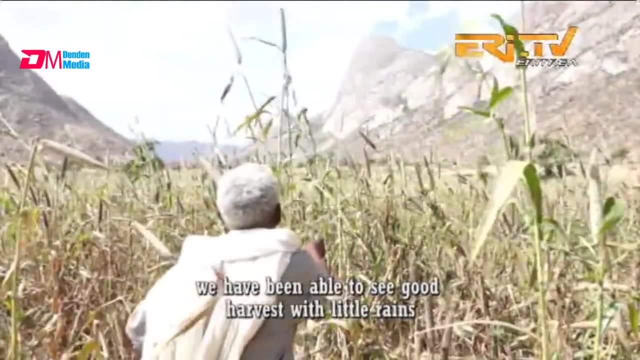 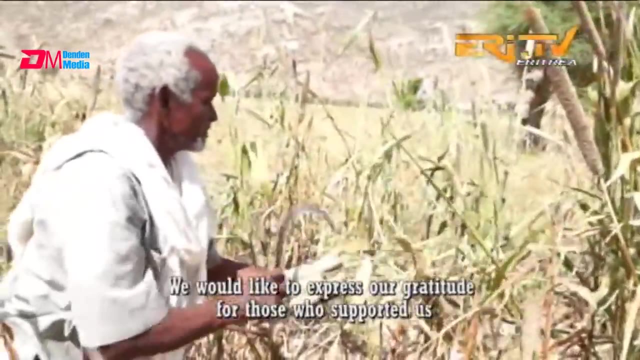 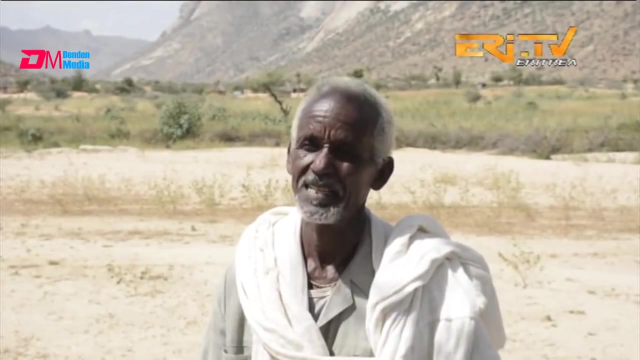 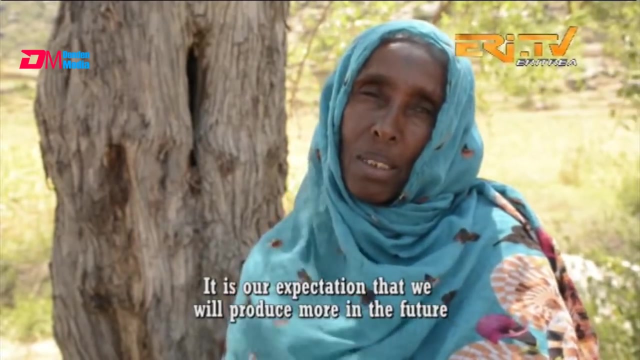 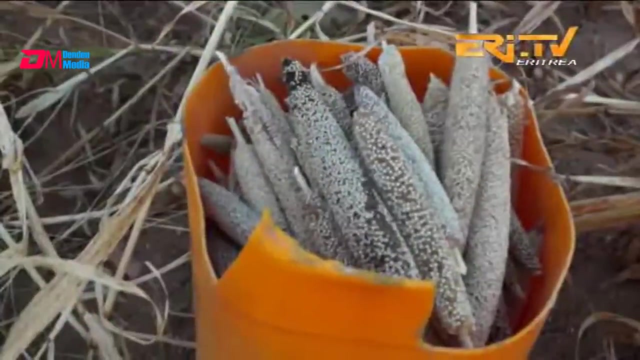 The program has been implemented in several regions. in the region, including the Jammu Kufu Kufu region and the Jammu Kufu region, We have already been involved in agriculture, agriculture and agriculture. These improved seeds distributed to these farmers are ecologically sustainable and climate resilient, and can yield more. 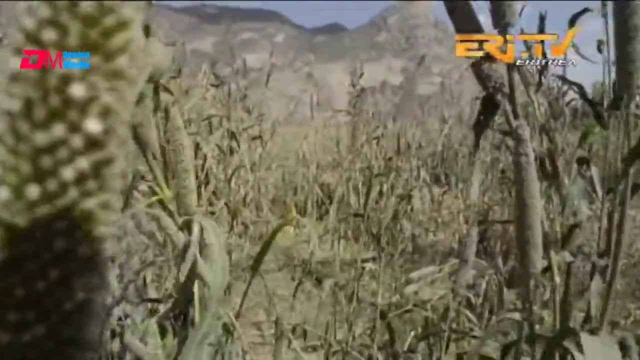 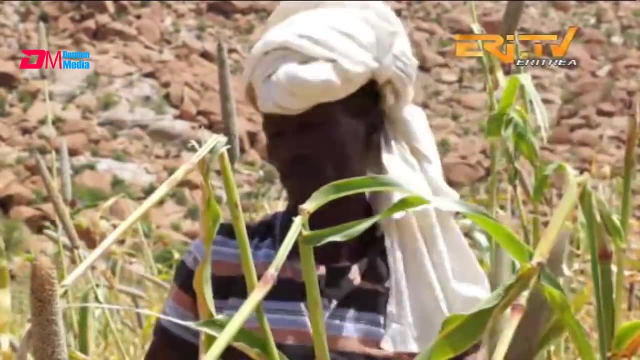 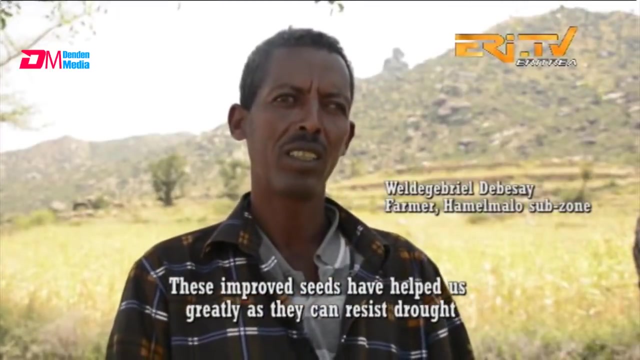 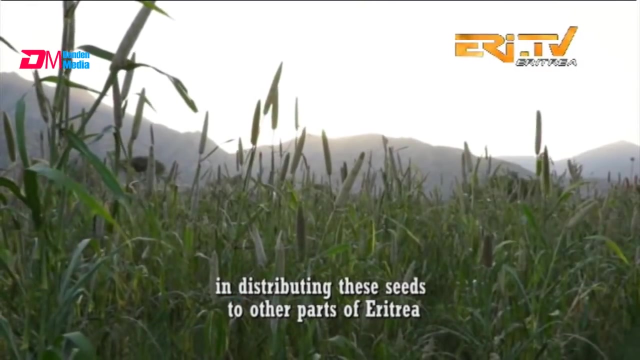 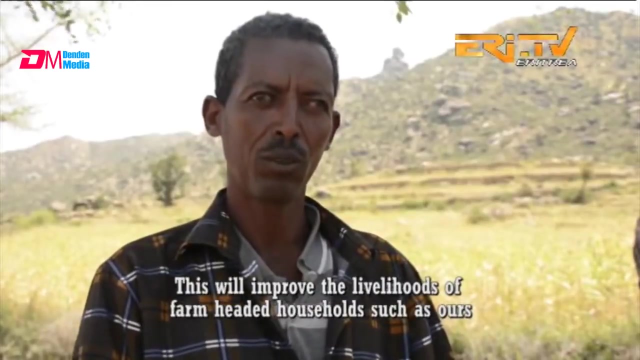 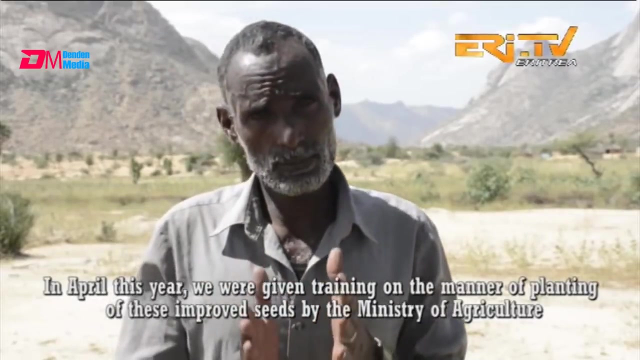 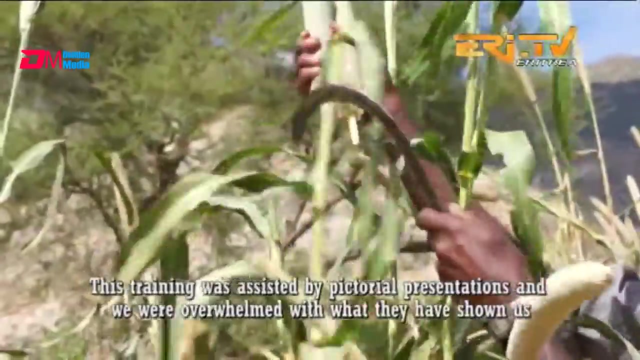 even in the dry season. Because of the distribution of improved seeds within the package of the program, many farmers are now able to plant crops twice a year, both in the rainy and dry seasons. We give you great opportunities to learn about the environment and the environment in which you grow your crops. I am now in a field that has 1,000 feet of land that I can see. It is in this field that I can see the land and the other land. 1,000 feet of land is an amazing land. I am very proud of it. 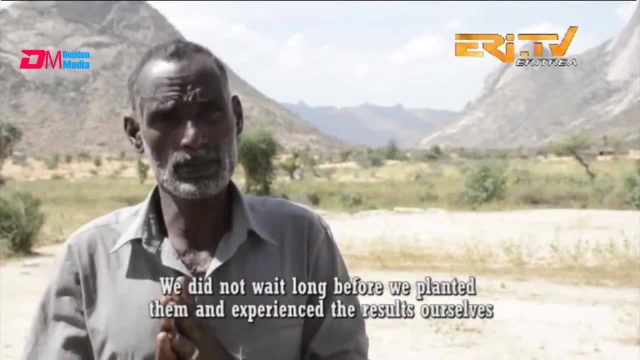 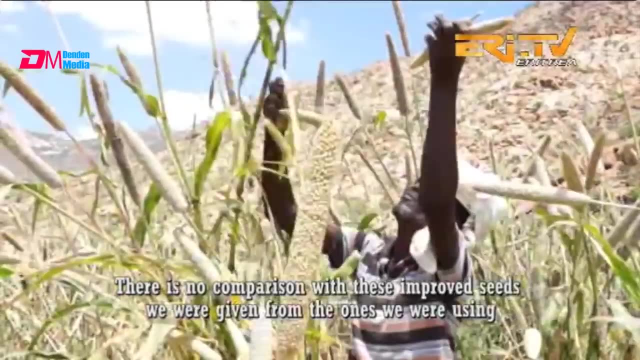 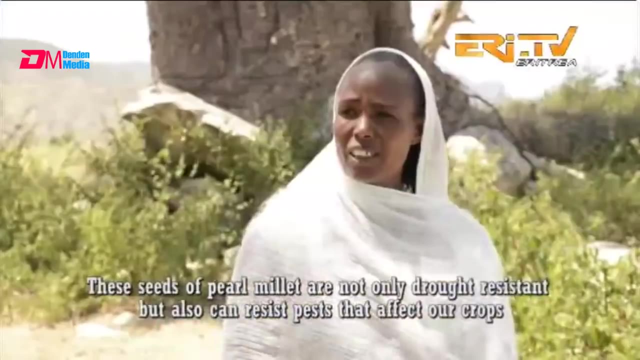 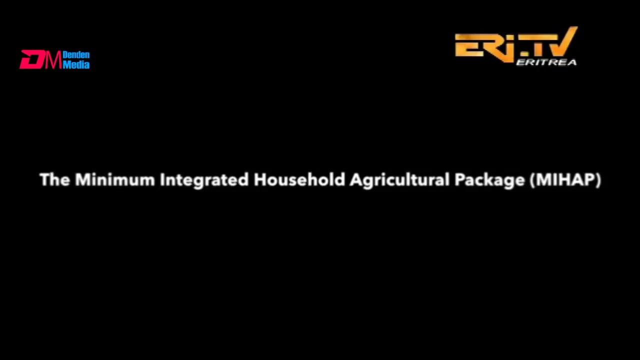 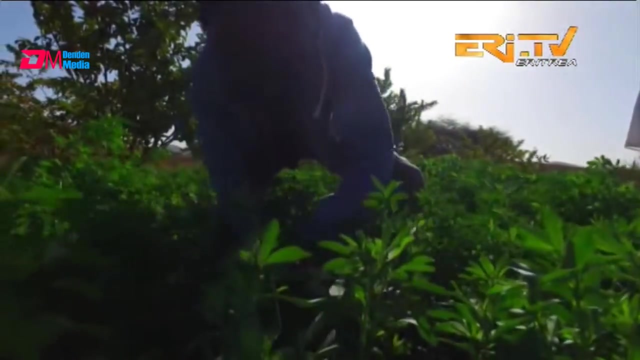 I am proud of it. If you want to see the land, there is only one way. If you want to see the land, there is only one way. The Ministry of Agriculture has piloted the Minimum Integrated Household Agricultural Package in complementarity with 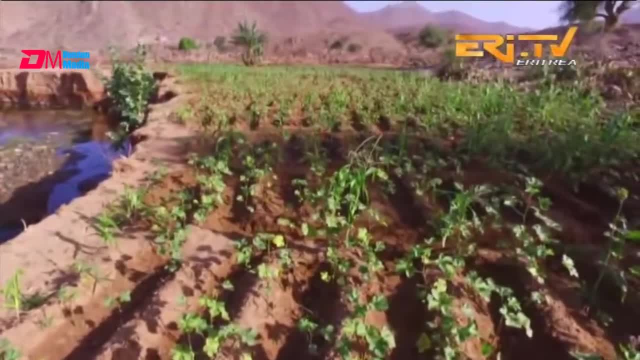 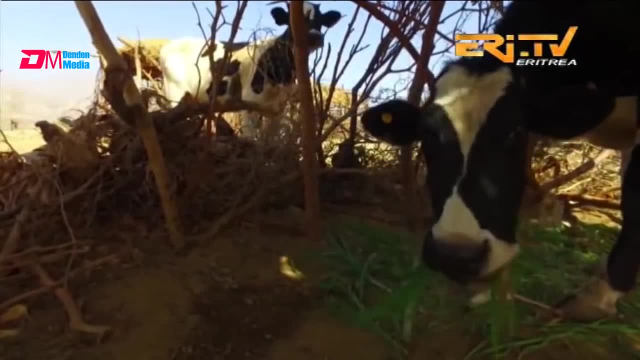 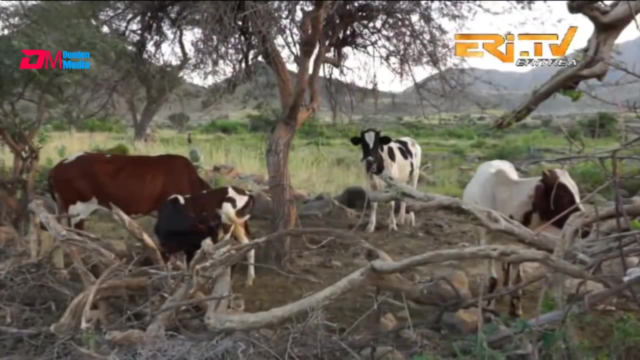 improved water availability. With the newly introduced Minimum Integrated Household Package in the Ansabal region, each house or family is given the opportunity to acquire one improved crossbred dairy cow or six goats. The cow is on a pass-on program, that is, the farmer gives back the first female calf of. 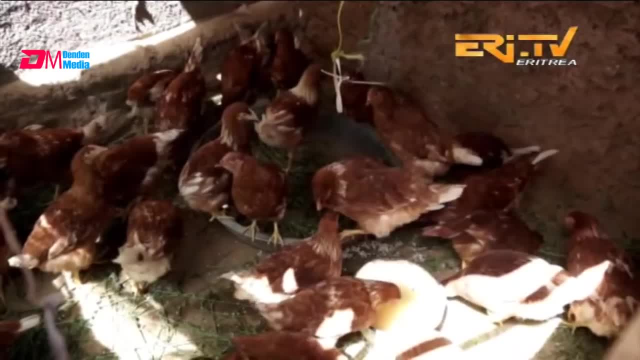 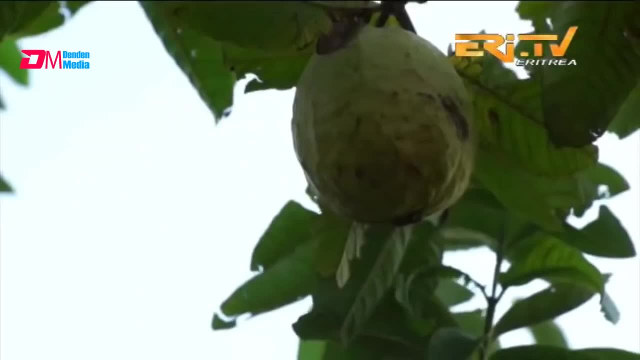 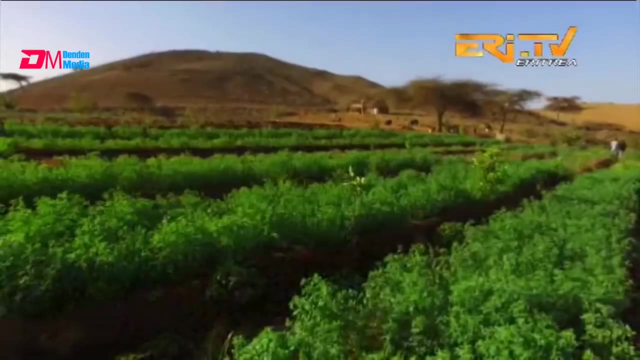 about one year. The package also includes 25 chickens, Only three of which are males, two beehives, a vegetable plot and 20 trees, 10 fruit trees, five leguminous trees as feed supplement to the cow and five trees for firewood. in addition. 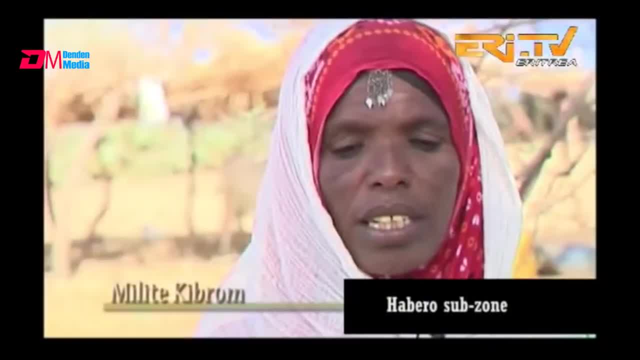 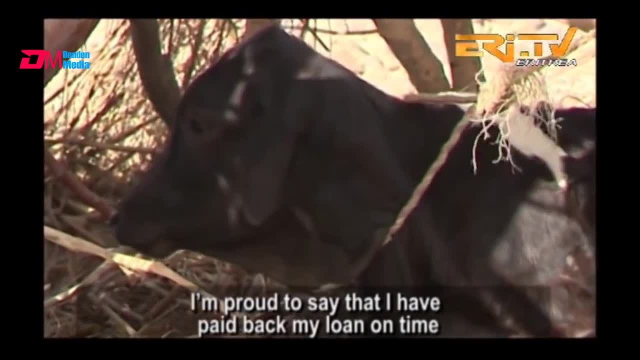 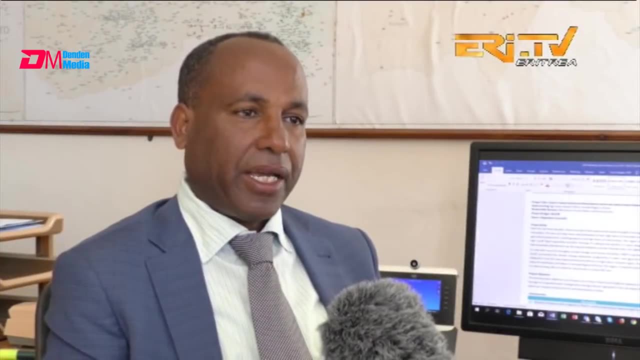 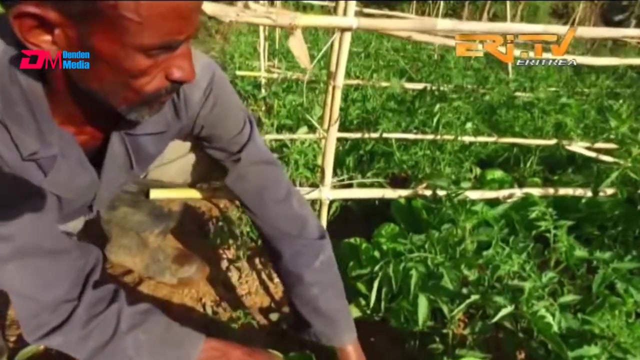 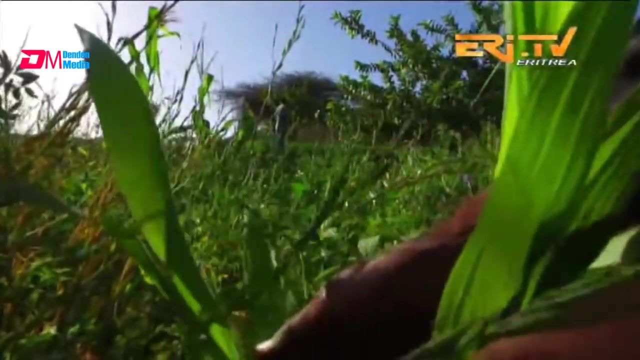 to the land used for crop cultivation, Training- all these packages is a packet. our intervention in that area is a packet. It includes water harvesting capacity of the farmers, training farmers on climate risk management and different types of agricultural practices. So all this led to improved practices for agriculture. 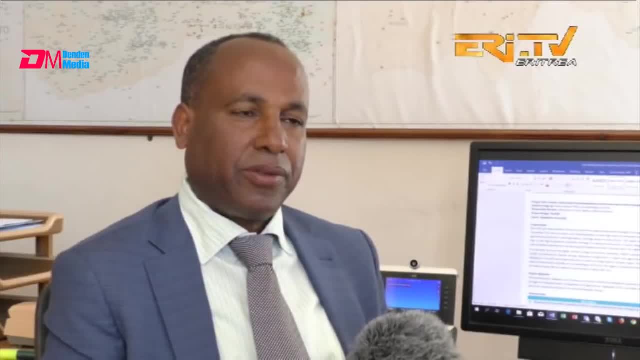 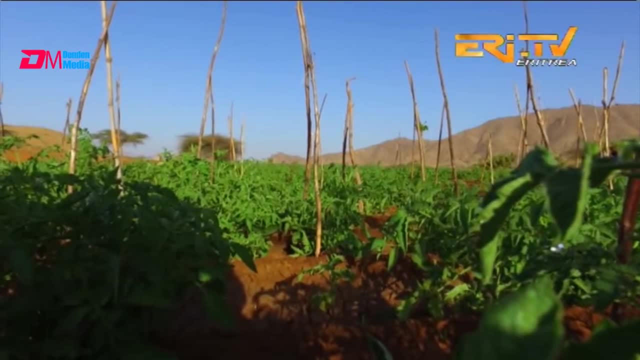 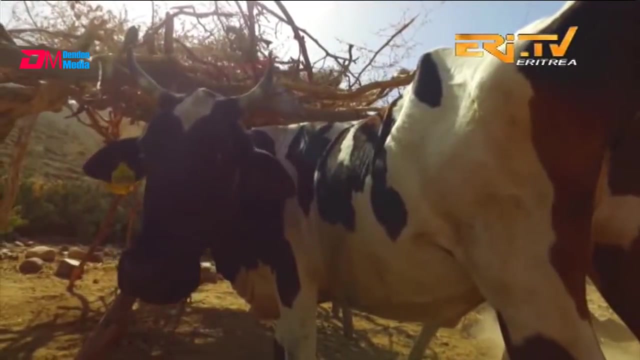 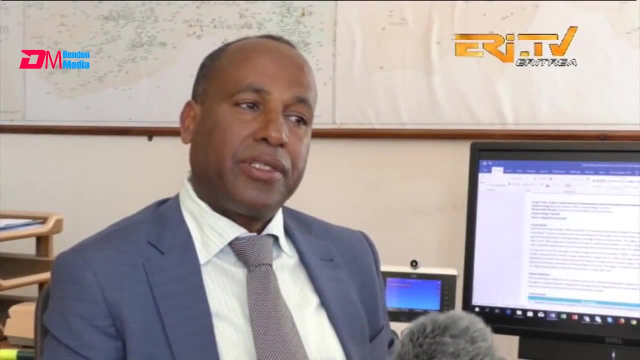 In that area so that helped farmers really to produce more, and by adopting improved management of natural resource and their livestock and crops. So it has led to improved livelihood in that area. This was realized through increased production of crops and higher productivity of livestock. 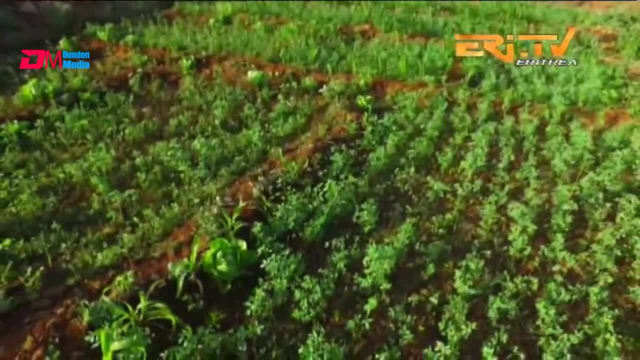 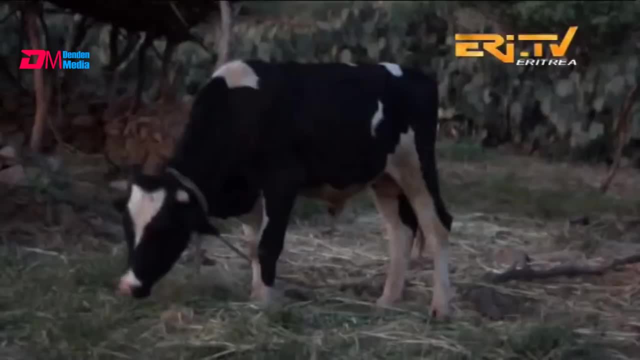 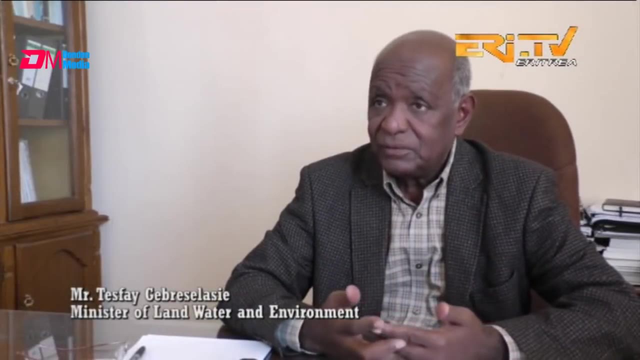 This approach has brought significant change in household production, food security and incomes. In fact, based on its success, the approach and package has been replicated in other development projects in the Zobar. The life standard has improved in terms of improving the quality of the food and quantity. 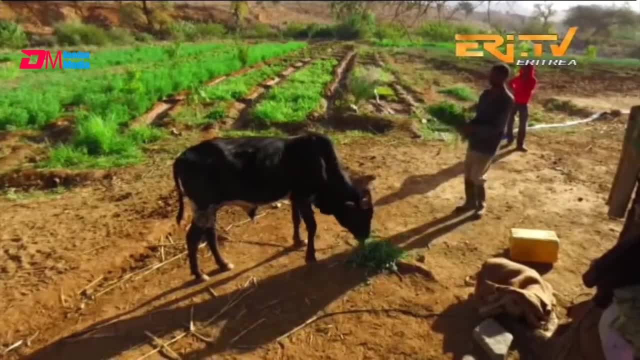 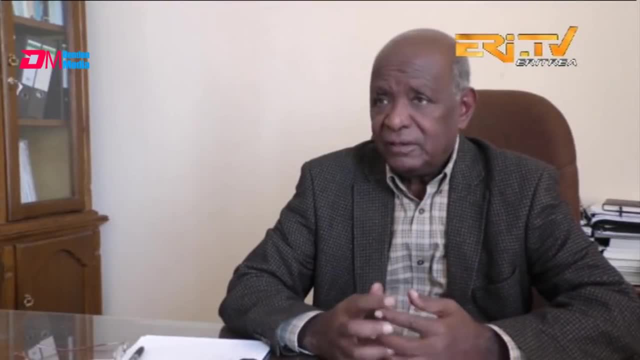 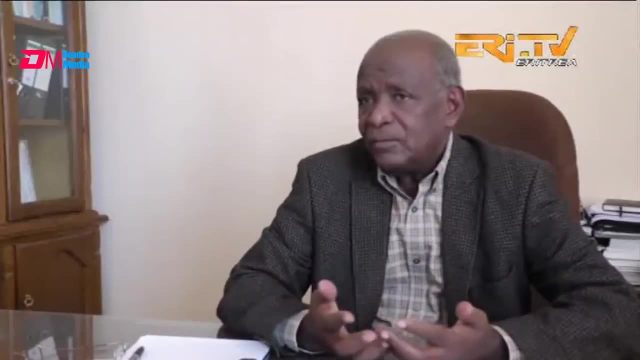 they get, And many of the nomadic households began to farm. So it's a good thing. It's a good thing The farmers now have settled their life and they are being engaged in agriculture- Before they were agro-pastoralists- and they roam around the areas in search of grass and 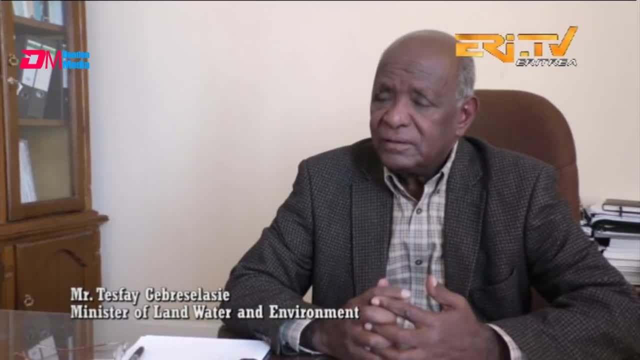 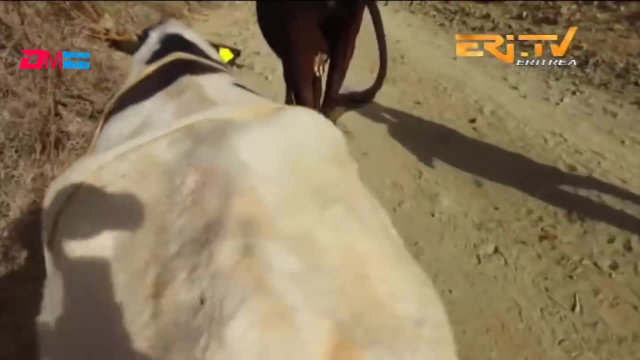 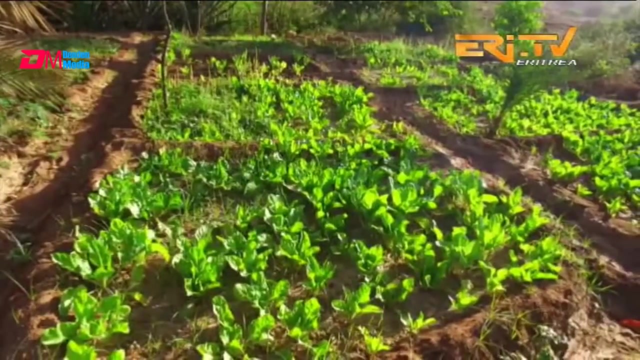 for their livestock. The distribution of crossbred cows, seeds and seedlings of animal fodder, fruits and vegetables has helped farmers improve the nutrition security at household level and supply market. They are now able to sell their produce in the villages and towns with milk animal feed. 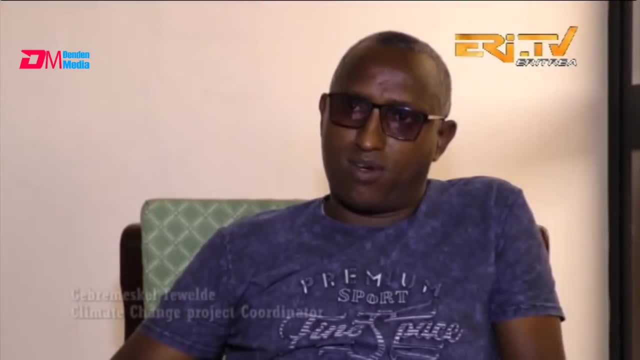 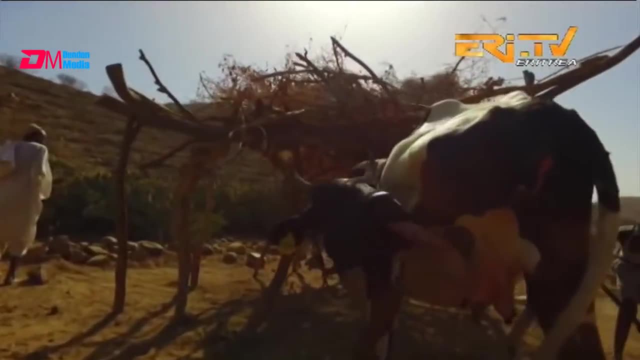 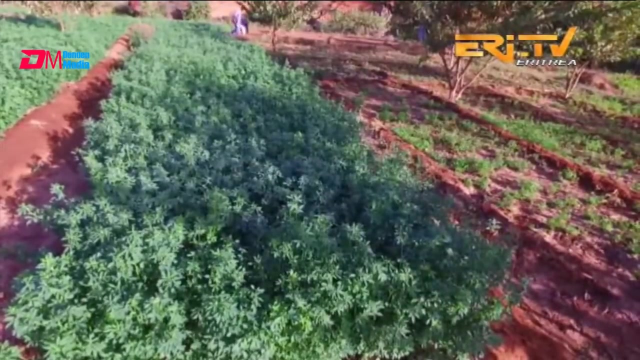 and vegetables at reasonable price. The main objective of this MIHAB to support the farmers to attain food and nutrition security, So this project assists them in provision of inputs and training and also in integration of these principles and ideas of MIHAB. 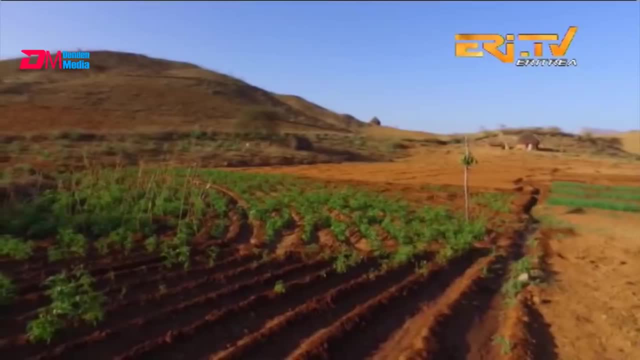 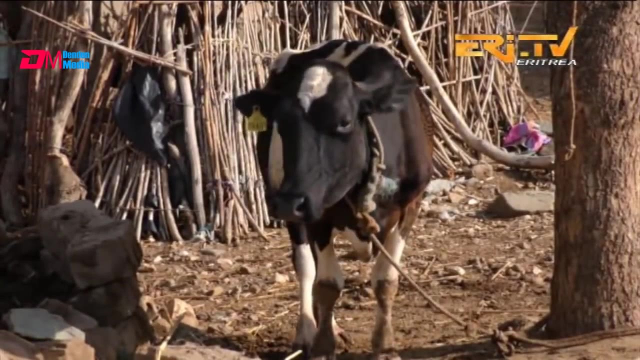 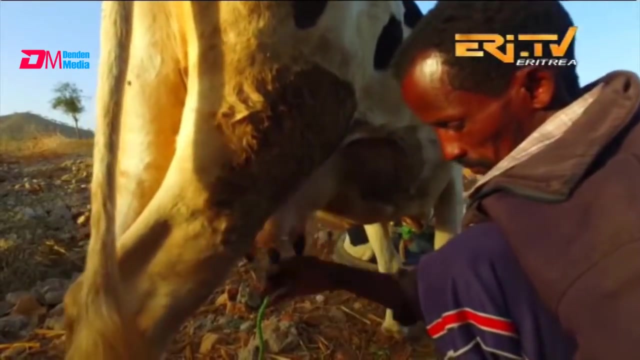 The program has successfully increased food and livestock productivity and hence food security. A farmer can now produce more than double or triple the amount of food they need for household consumption. Similarly, milk production has increased from 2 liters per day to about 5 to 8 liters per 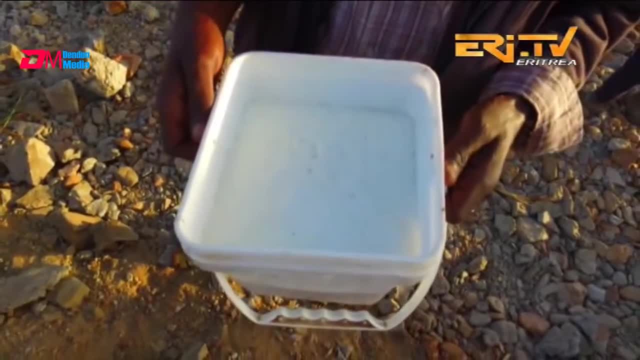 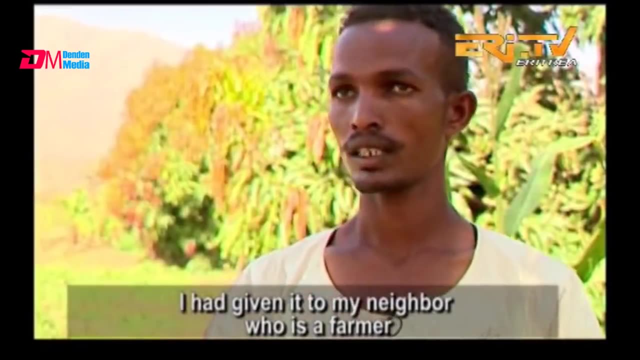 day and the excesses are taken to the markets for sales to generate household income. We've been working for a long time to start doing this. We've been working for a long time and since its last year, we've been working for the next. 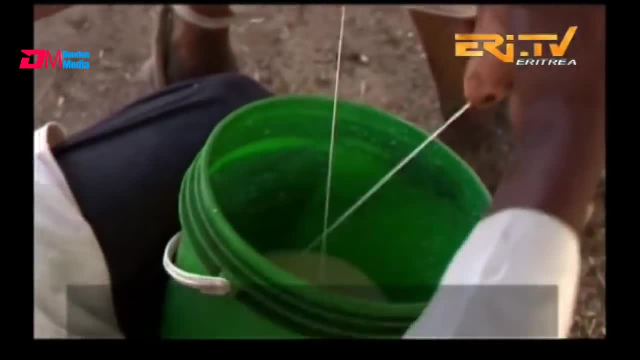 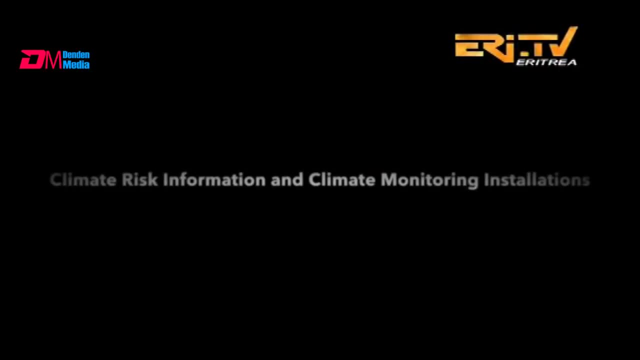 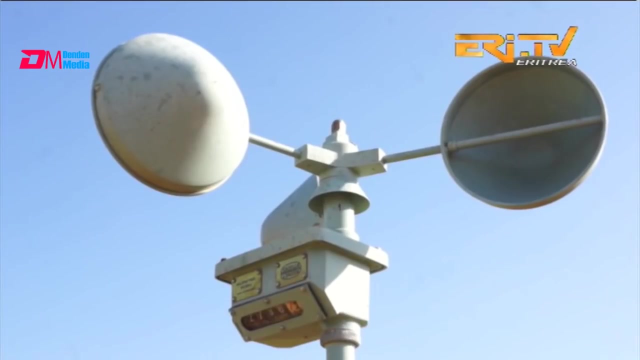 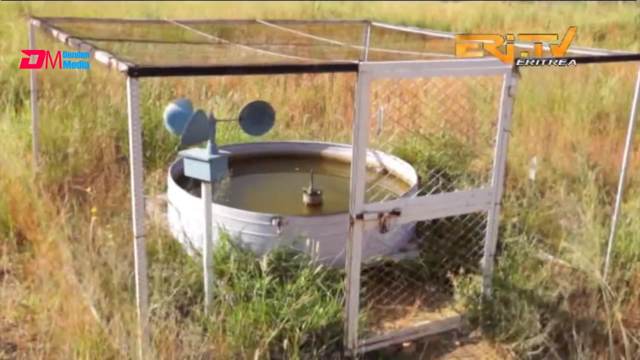 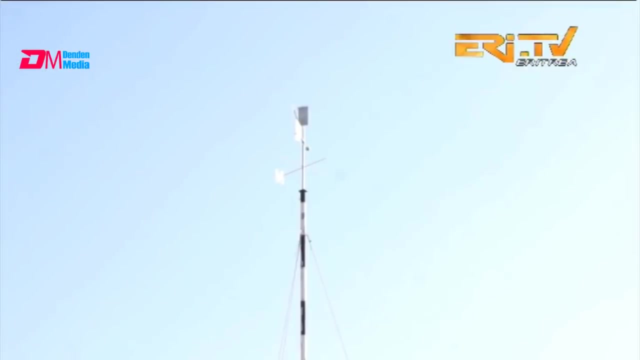 year The project has installed six meteorological stations in the Ansaba region to enhance community preparedness to climate hazards. These installations at the Hamel Malou College of Agriculture and the Agrotechnical School have provided access to students and faculty to conduct training and research for improved 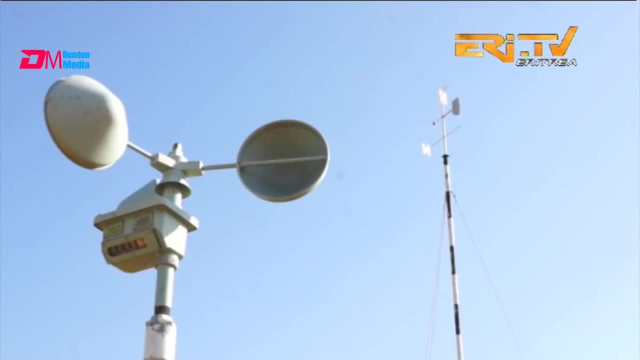 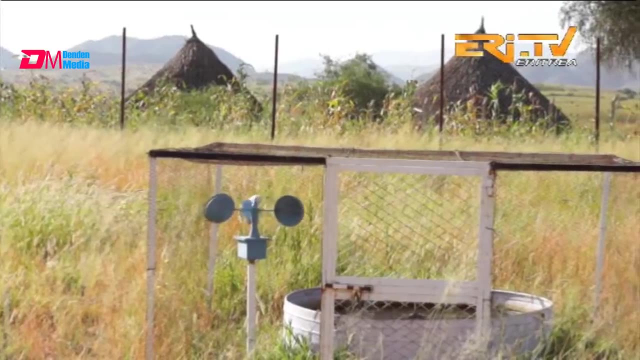 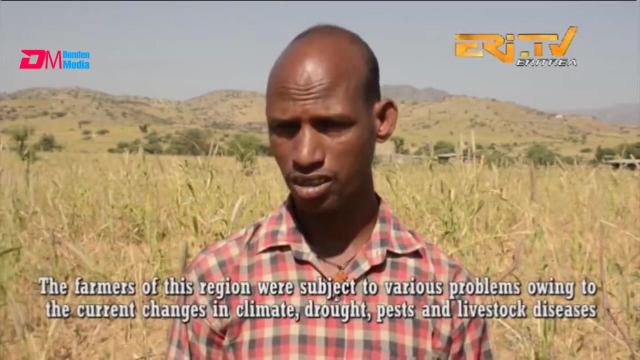 weather forecasting. Also, the data generated from the manual stations is being shared with the Ministry of Land, Water and Environment and the Department of Water Resources. We want to make sure that the environment is safe for the people who live in the area. We have to make sure that the environment is safe for the people who live in the area. 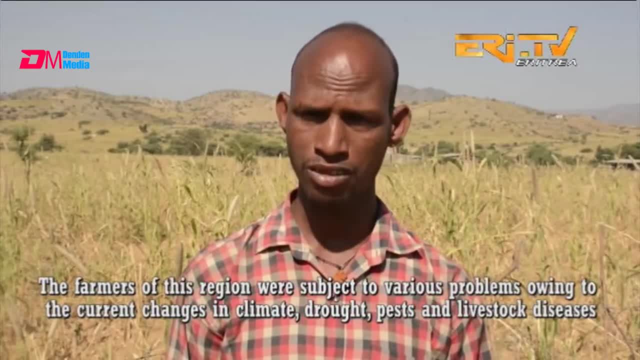 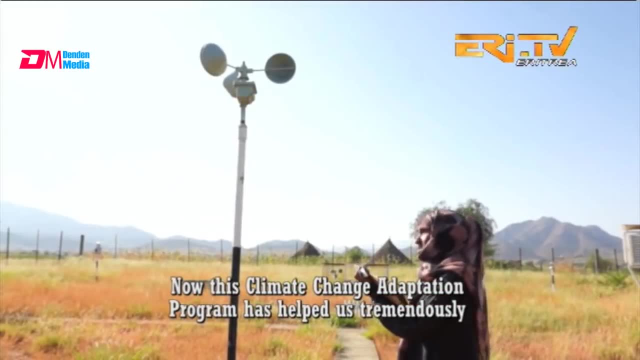 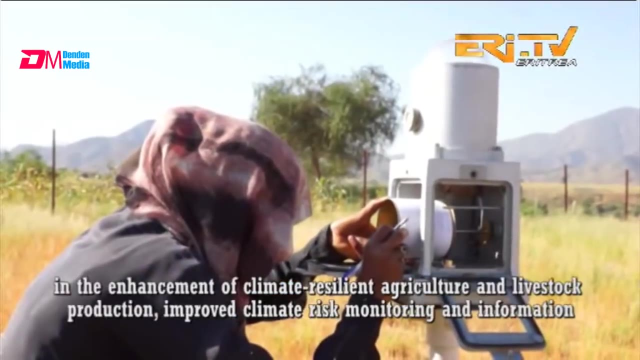 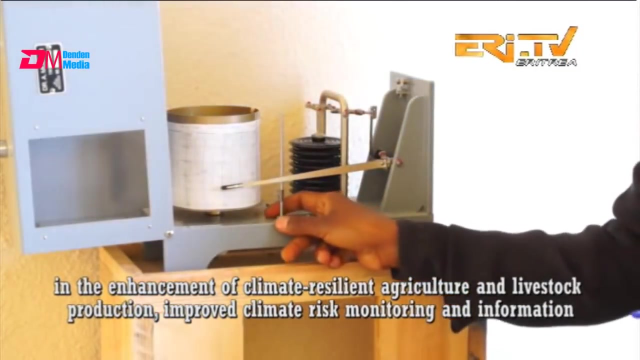 We need to improve the environment for the generations to come. We want a safe and secure environment. Will this be effective? Yes, if the city had suitable conditions instead of dosing use of water. supposed to slow down the consequences of climate change through Kwabirud. 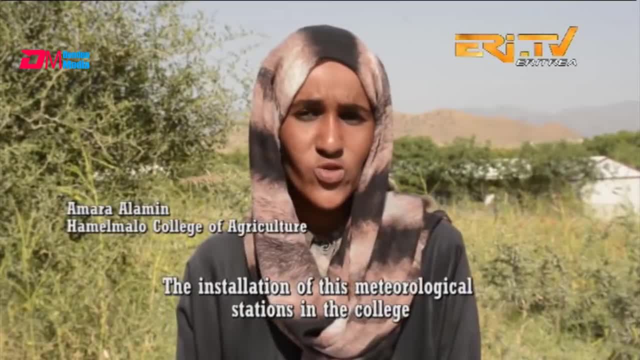 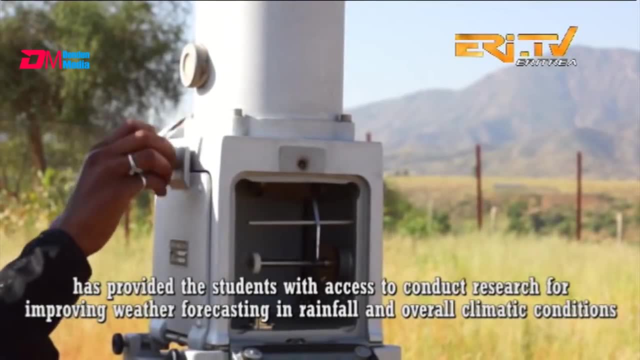 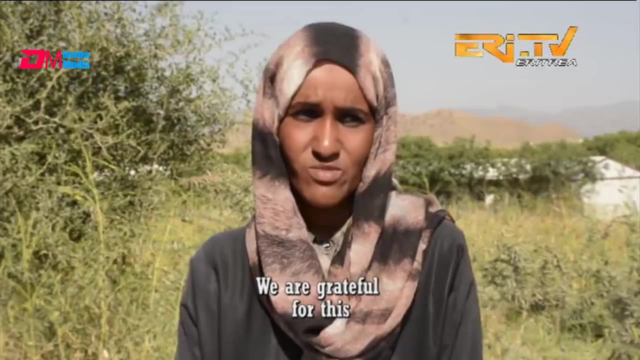 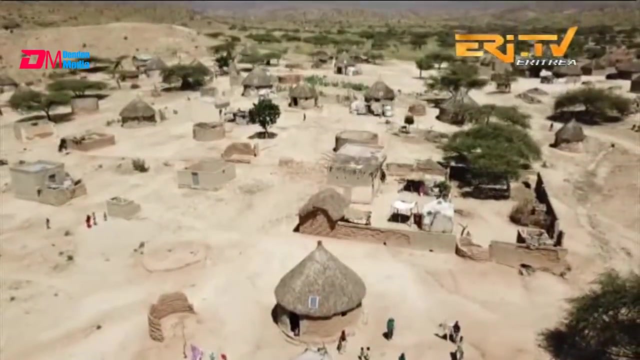 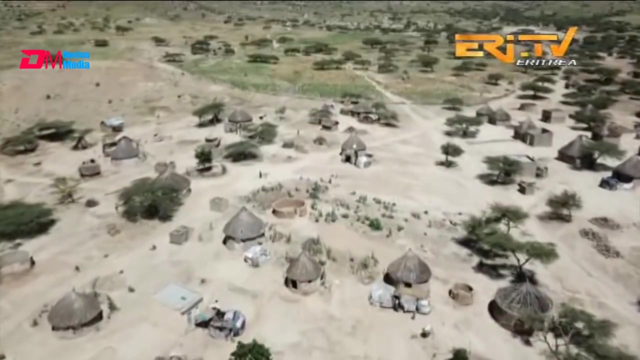 It has been time consuming. Are you confident? Due to its high priority to the community of both Habero and Hamelmalu subzones, solar panels were installed in 748 households. In addition to its climate mitigation benefits, this intervention supports the farmers in 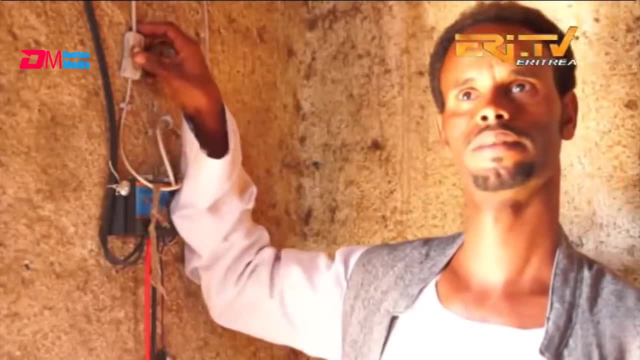 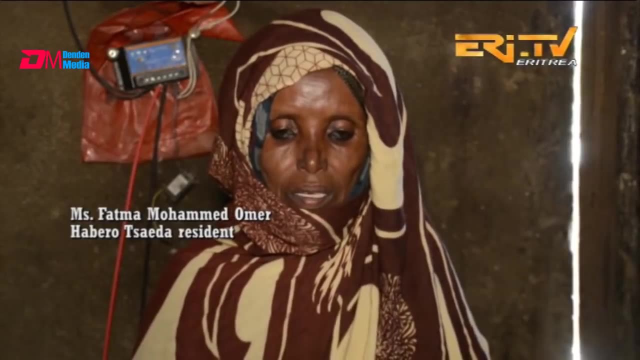 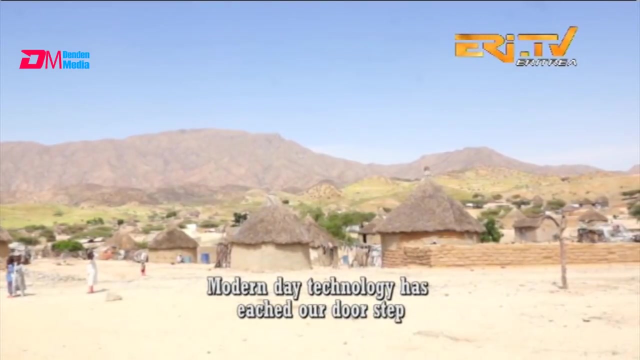 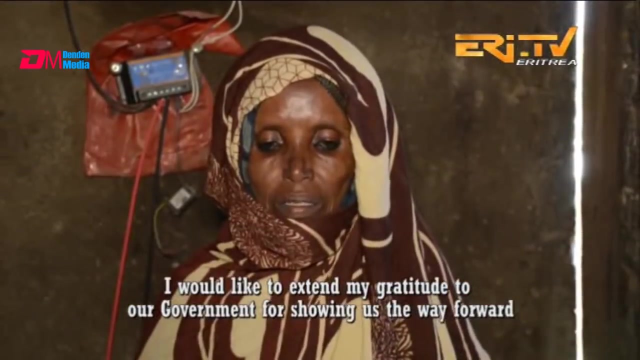 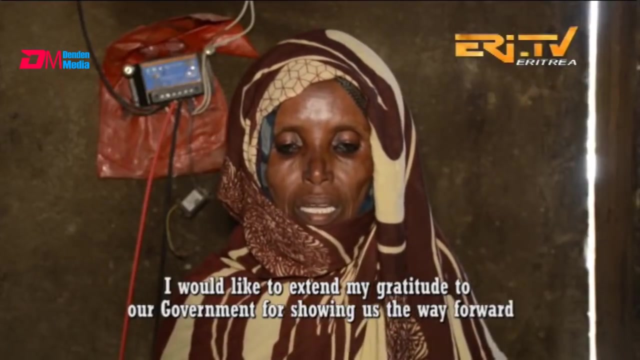 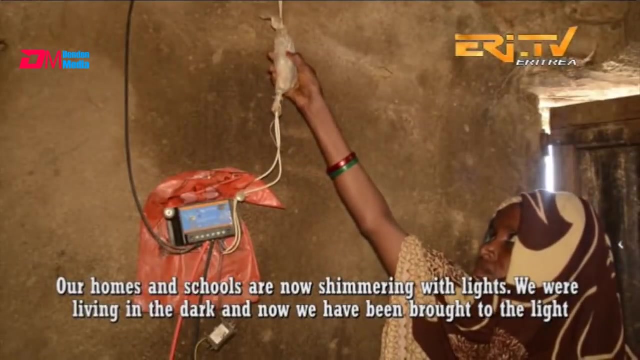 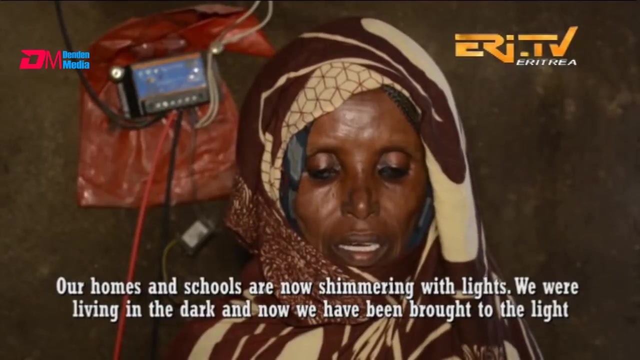 upgrading their house income by minimizing household expenditures on purchasing of kerosene. Good morning everyone. we are the farmers who are helping this country, our community, our neighbors and our family. We are having a great time here in this community. we are celebrating the holiday here in this. 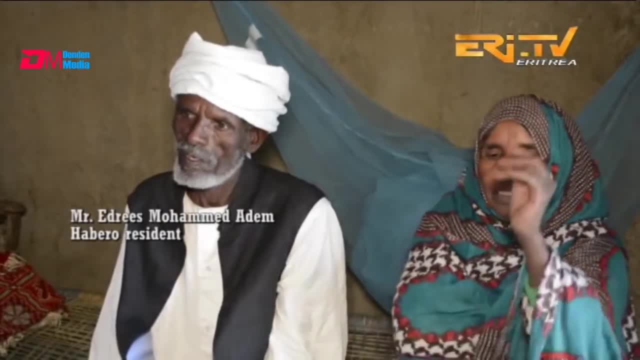 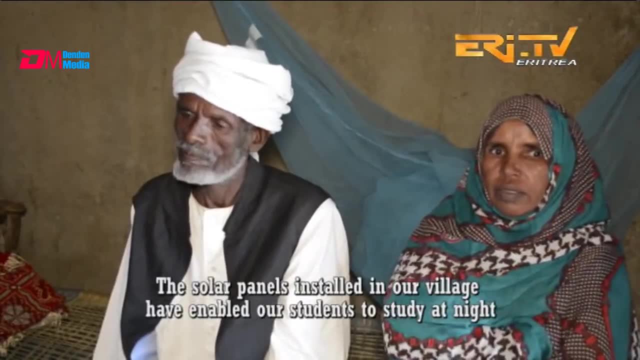 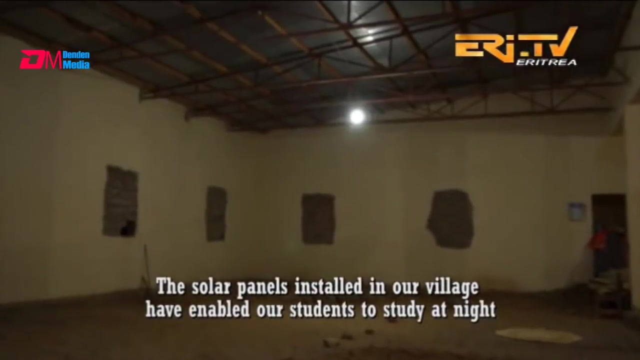 How many people are still living in the area? We have more than one thousand people with the current situation. We have a lot of people that have passed away. We have a lot of people that have died in the past, but we have a lot of people who have been killed in the past. 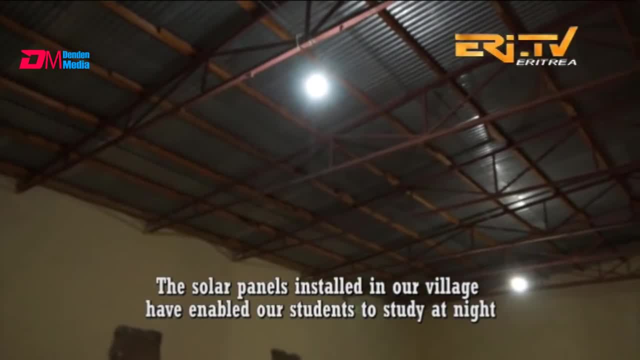 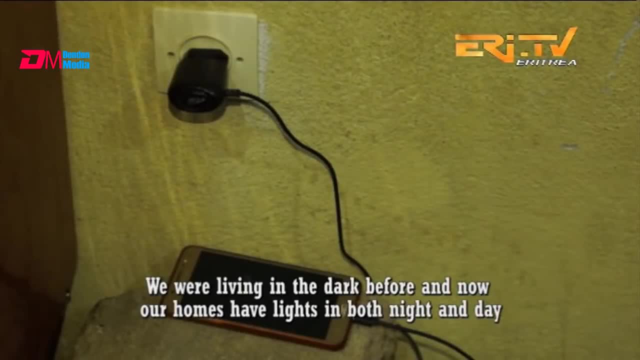 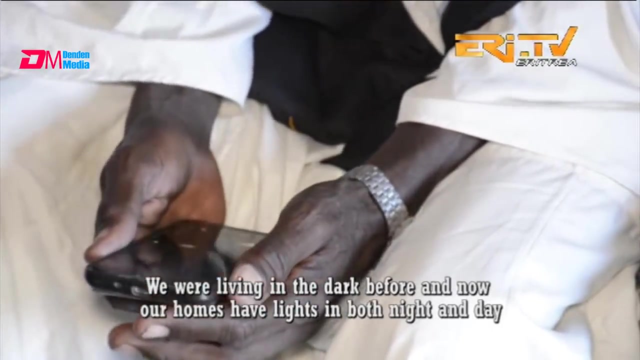 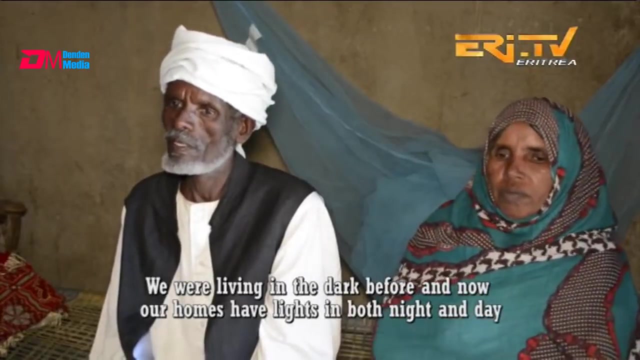 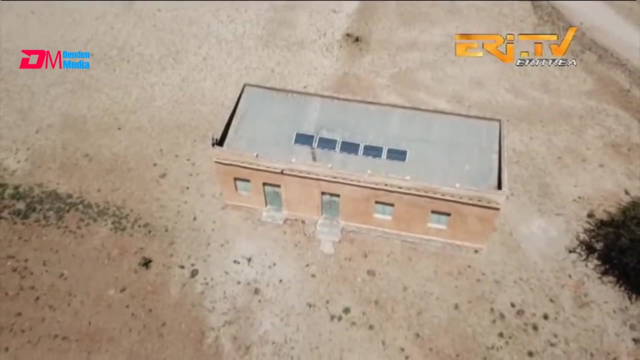 We have many people who don't have mobile phones and we have people who have lost their homes. We have a lot of people living in the area. Since three schools are also benefiting from the solar lighting, the intervention had contributed in improving education in the society. 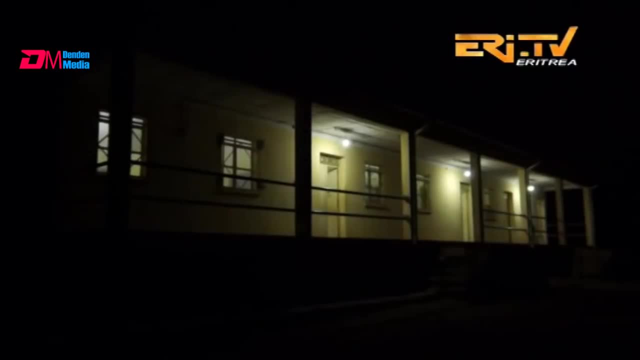 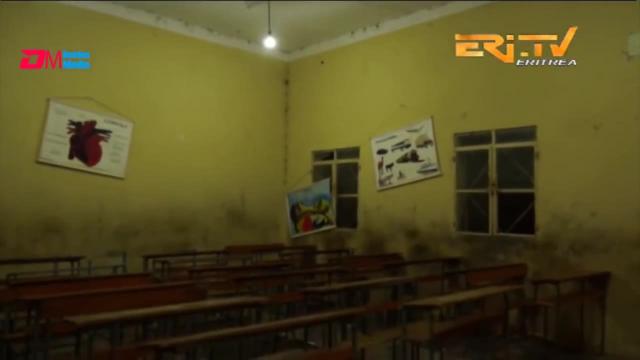 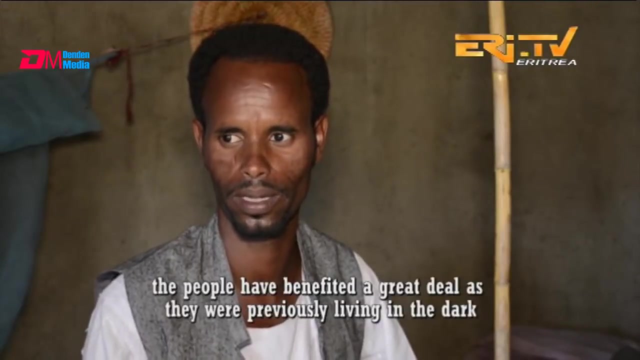 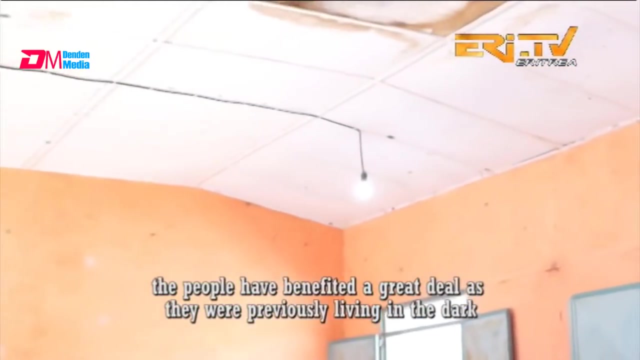 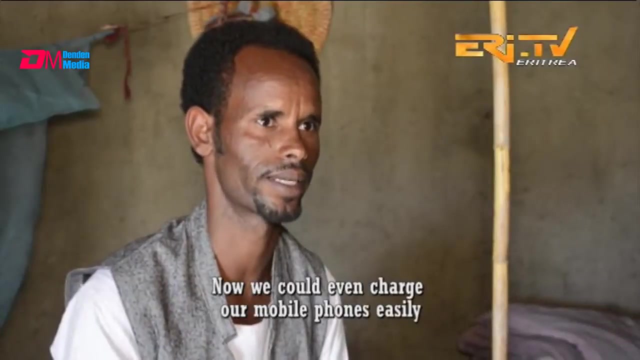 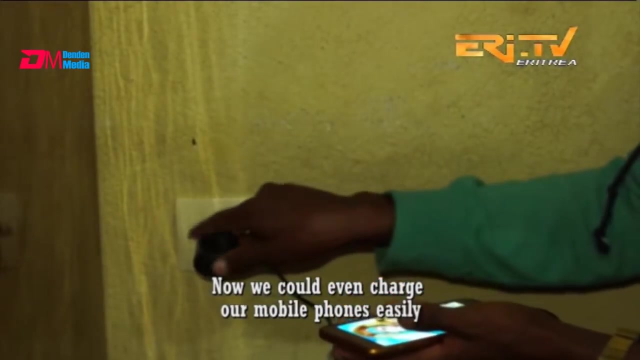 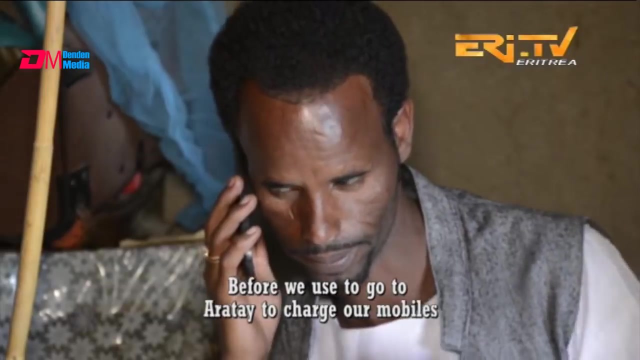 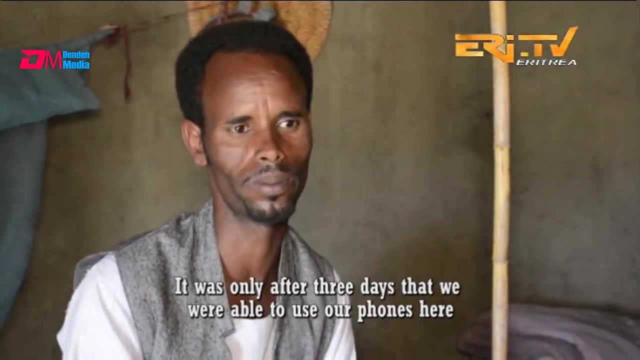 by giving opportunities for night studies and using some electrical or electronic tools, such as computers and tablets. In the past, we used to use mobile phones to charge our phones. Now we use mobile phones to charge our phones and we can charge our phones at any time of the day. 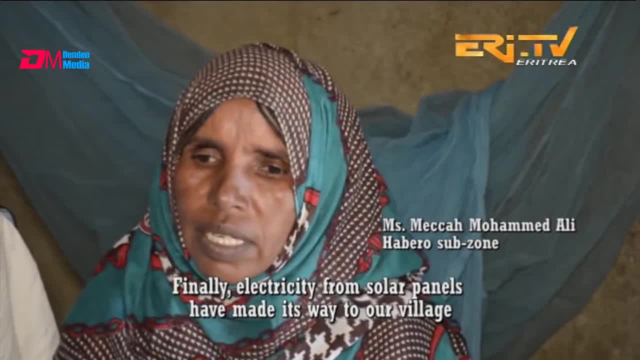 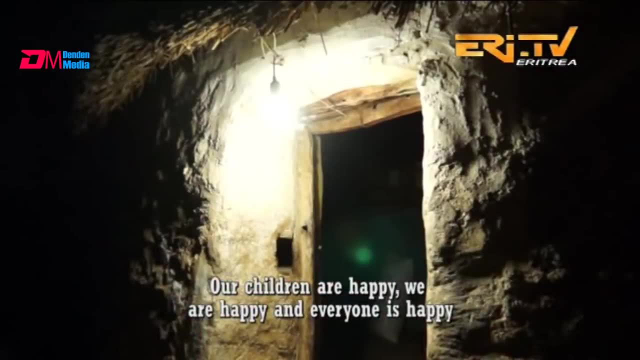 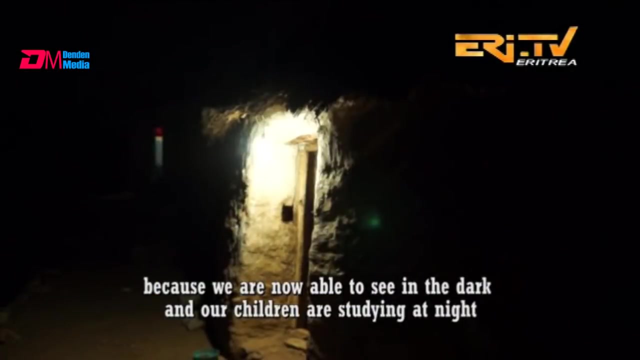 Thank God for the light. Thank God for the light. Thank God for the light. We hope that the results will be real and that our mobile phones will be set free as well. We promise our lives to God, but if God wants to seduce us within 250 days, we will not. 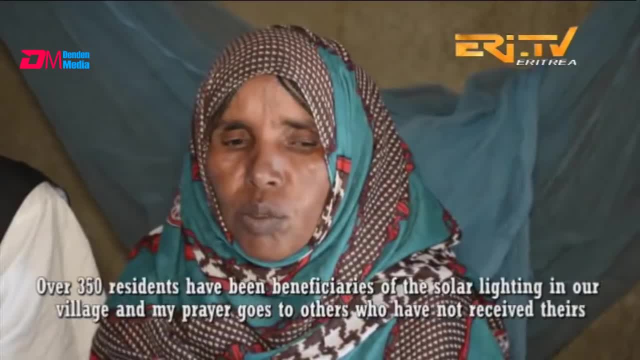 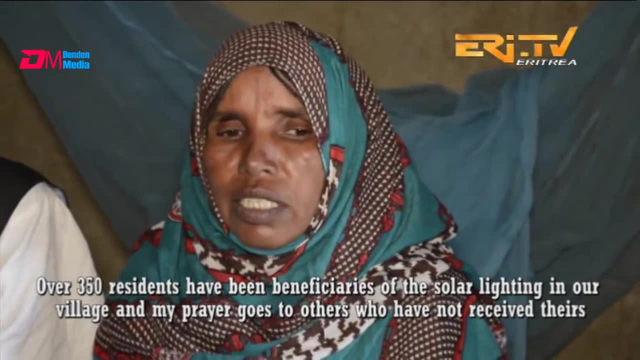 and if God wants to, He will, just like He promised us. He promised us all of this, so we will be happy And thank God. God knows that we will be able to live our our lives and we will be able. 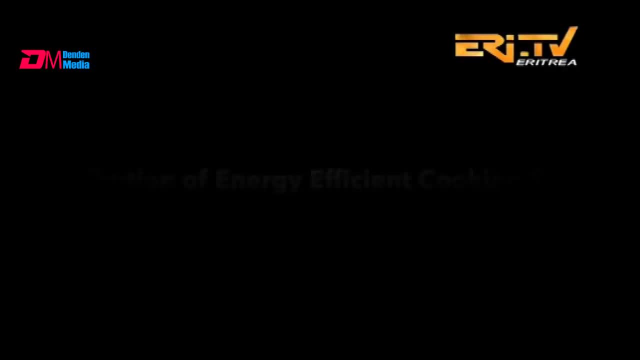 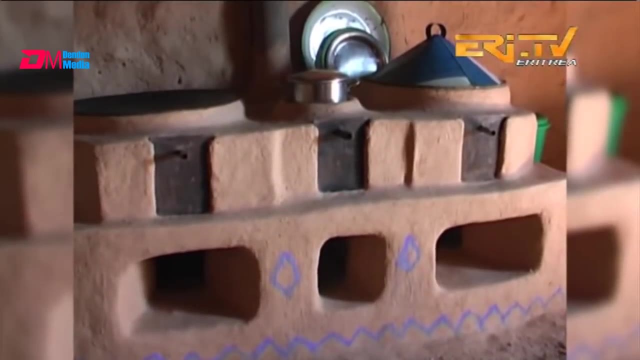 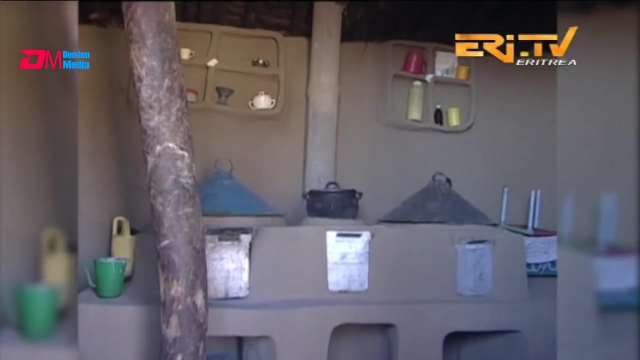 to be happy. About 1,700 women-headed households have benefited from the distribution of energy-efficient cooking stoves, which not only reduce fuel utilization and play a huge role in decreasing deforestation rates, but also play a positive impact on women's health. 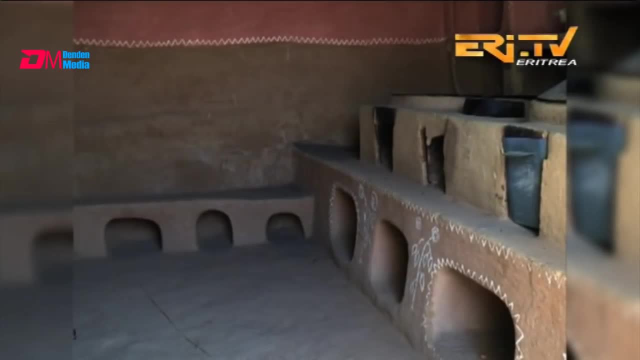 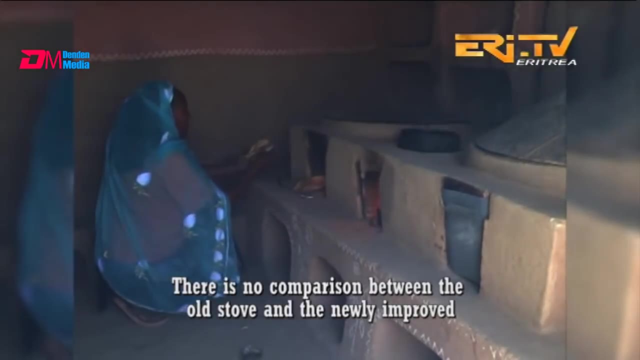 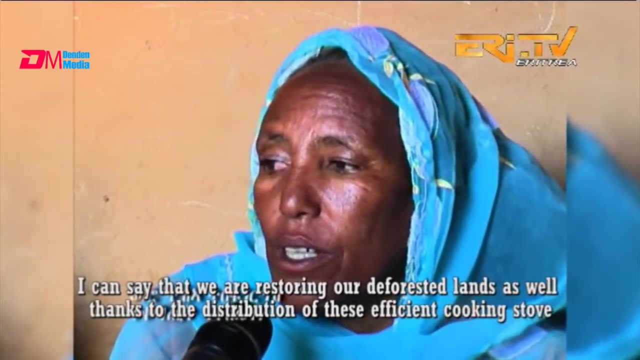 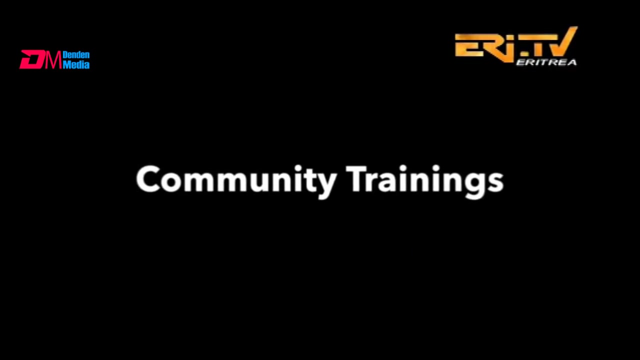 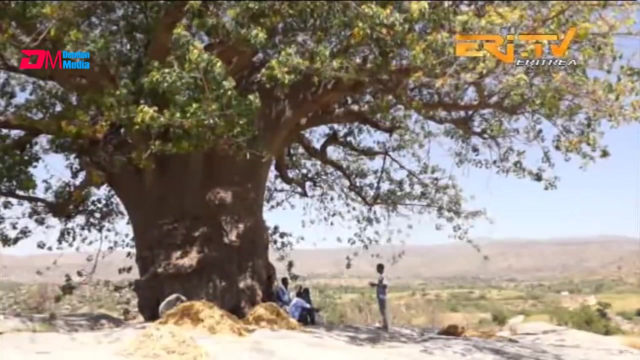 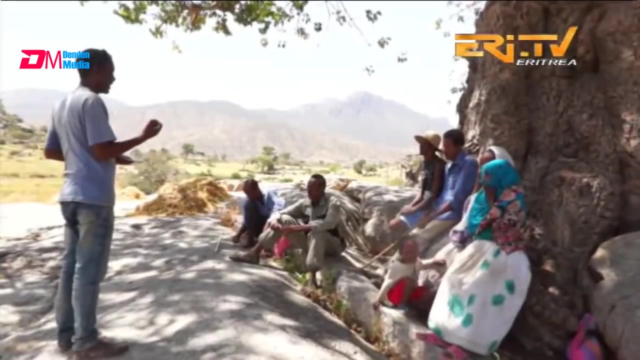 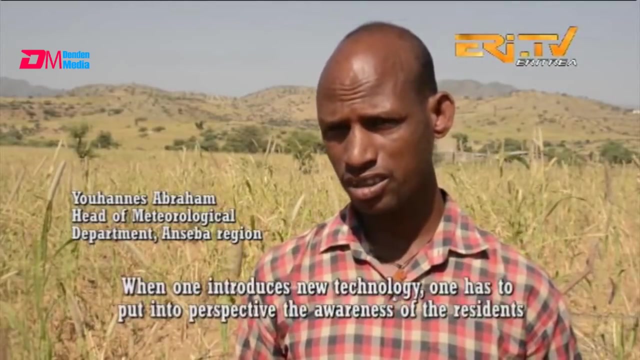 and the efforts to gather timber for basic household needs. Several farmers are given trainings on animal production and health, fodder cultivation, horticulture and irrigation, establishment of the dairy farms, cultivation of fruits, animal feeds and vegetables. The technology that we offer is very advanced. 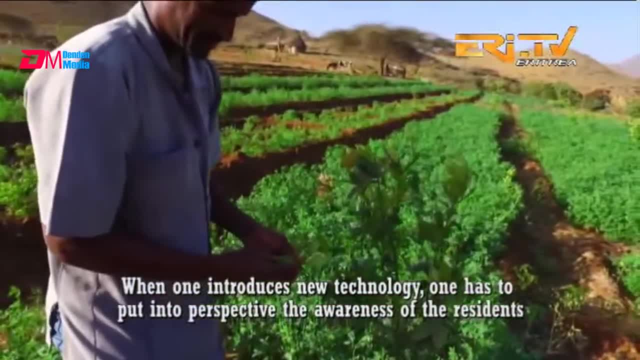 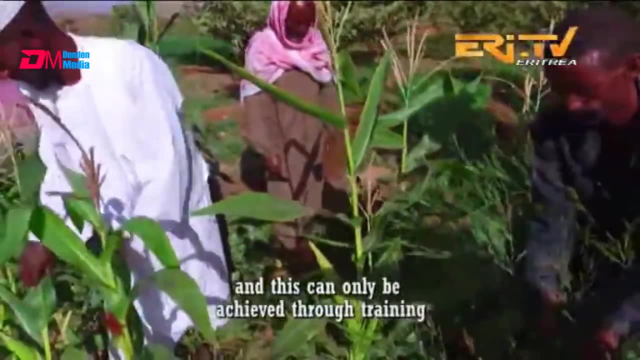 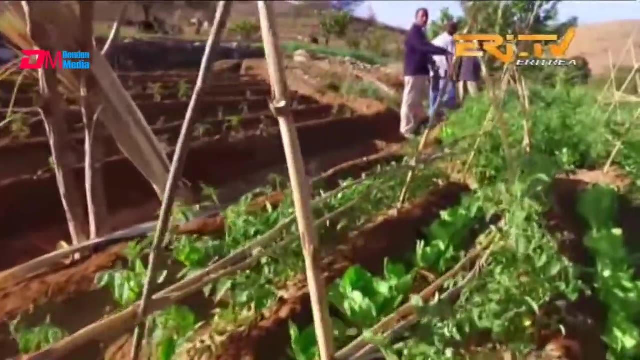 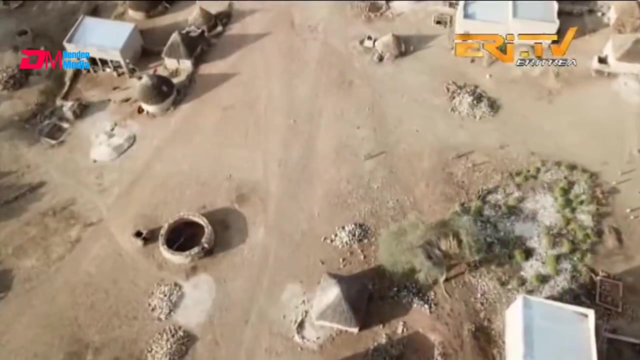 We are very careful with our awareness. We are very careful with the equipment we have. We are very careful with the equipment we have. We are very careful with the equipment we have. The program has directly benefited over 6,000 households, including 22% women-headed households. 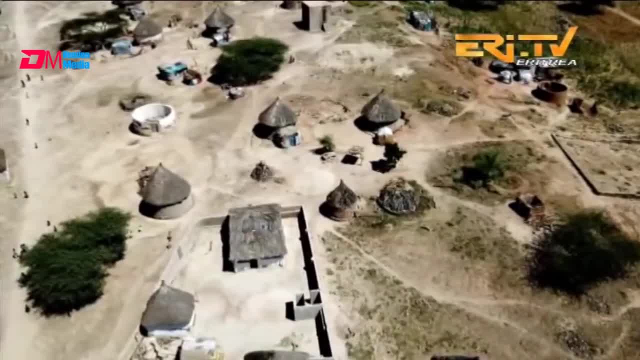 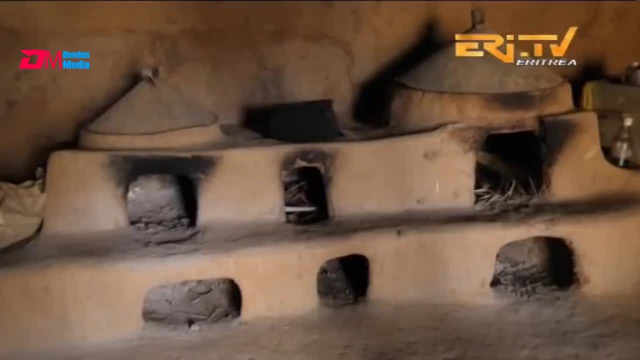 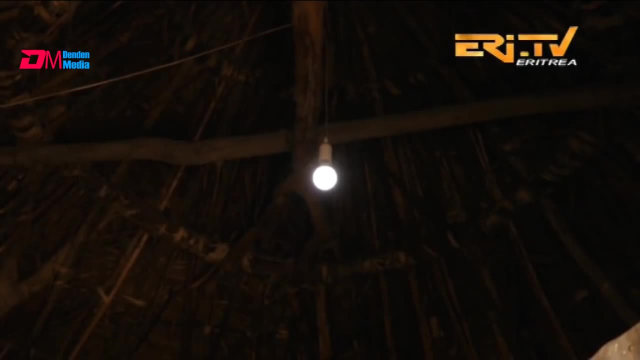 and indirectly directly benefited over 75,000 inhabitants of the two subzobas. The Minimum Integrated Household Agricultural Package, coupled with traditional, improved fuel-efficient stoves and solar panels, provided diverse livelihood options and opportunities to many farming households. יה تىّ سرِعهْ …. 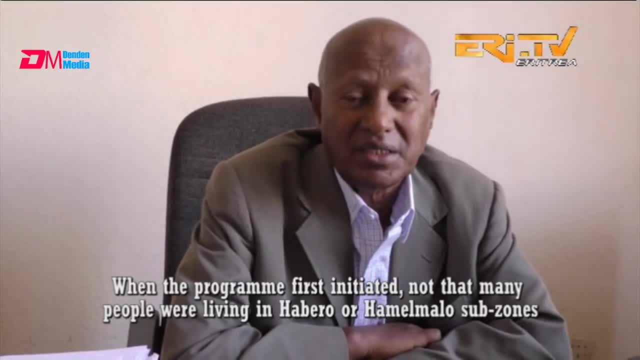 كجمّر کُدلّو وب behaving in Itraaj, that everyone is treated like a friend. قدُفِلّٻا حبّر aquí數ات ساوات يعن بارون, then it is better to engage as much. 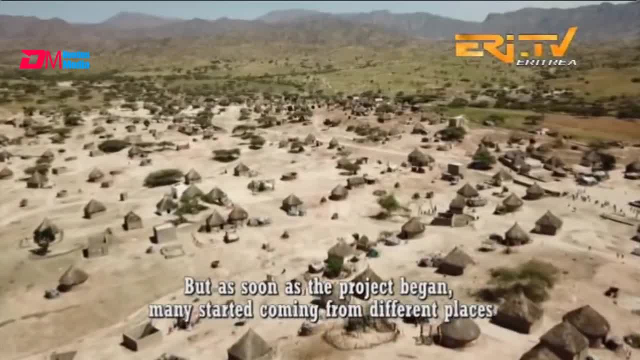 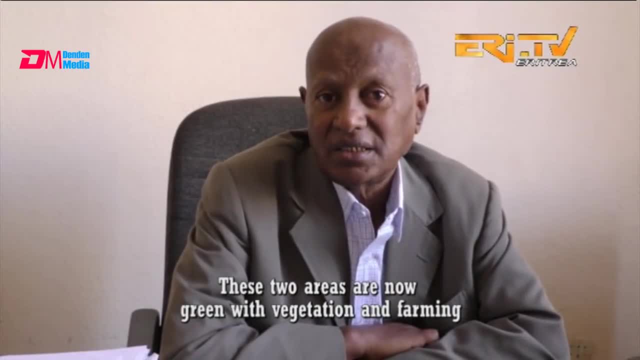 السّ+ psic—الحد, frozen in Irkutsk and was woven. in the process, we improved it greatly. جمّر،RYUNG… pri者،بوطّا nozzle adiocontrol, comedām laid diipotā. 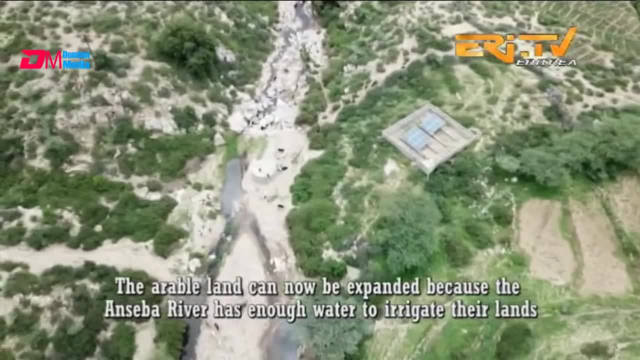 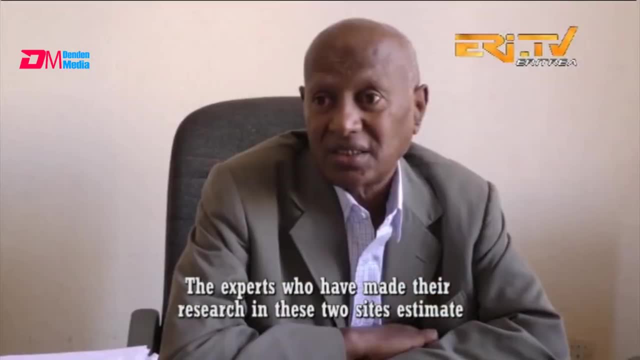 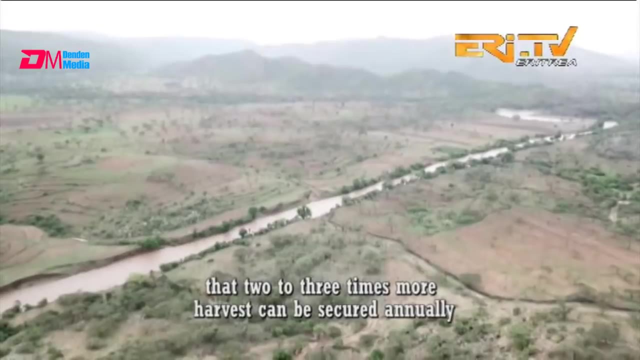 Les êmiru زیادا añadfer 음 coses. We were able to go to the airport and visit the country on the last day. We were able to not only visit the country, but also to travel all over the world.